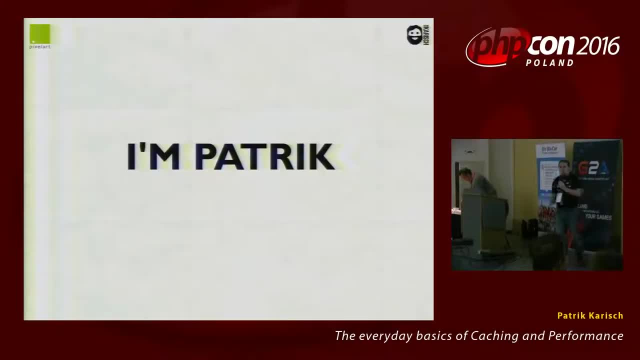 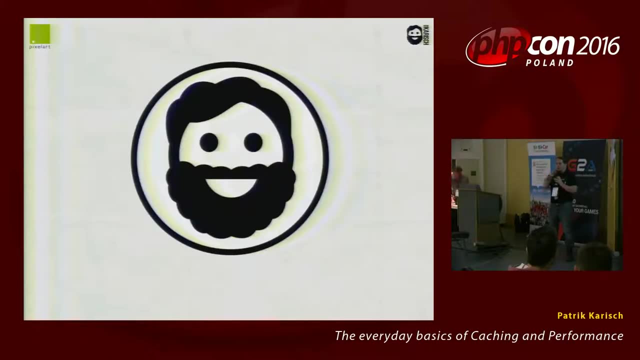 First, hi, I'm Patrick. I'm a back-end developer, mostly PHP. I hate JavaScript, to say it, And this is me. I am on GitHub, This is me on Twitter, This is me on Keybase. This is me everywhere. 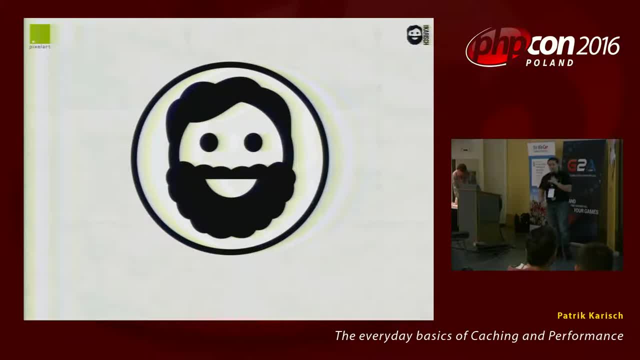 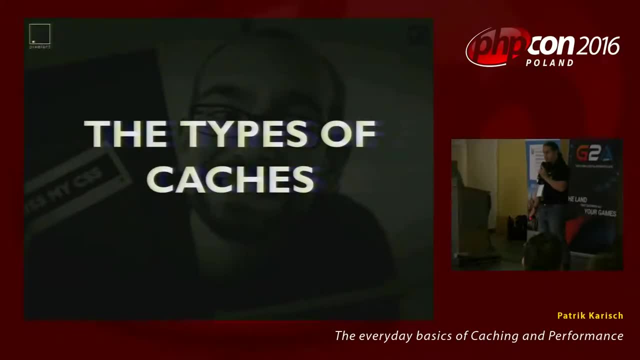 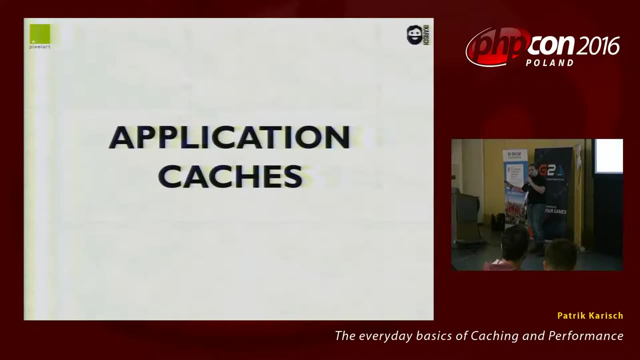 It's not accurate enough. I have shaved too much, But this is me. Remember it. Today. let's look at four different types of caches. First for you, I have the application cache, And if we go further from the application, you have a gateway cache, or better known as a reverse cache. 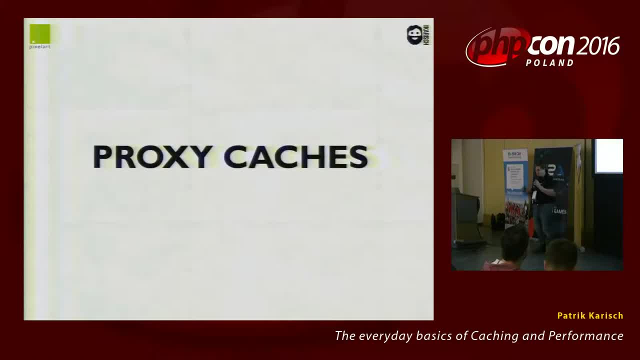 Or then you have the proxy cache- annoying stuff- And at least you have your browser cache. Who has ever made an application which uses the browser cache? One Never used the browser. Two, three, four, five, six, Okay. 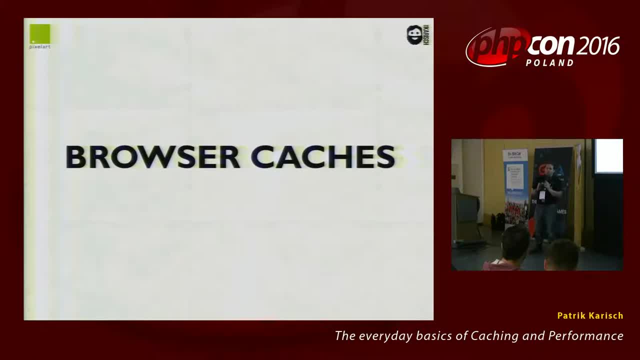 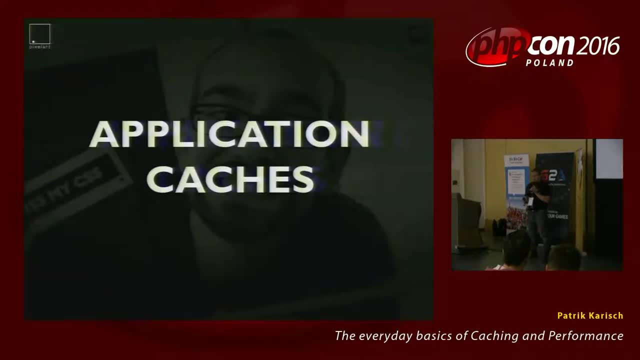 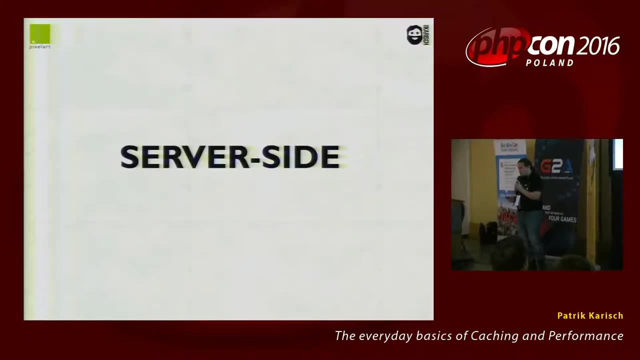 So some of you don't have forgotten the browser cache, but most of the time it's a forgotten topic. But let's start with the application cache. The application cache is really important for you because it's on the server side and you have the full control of it. 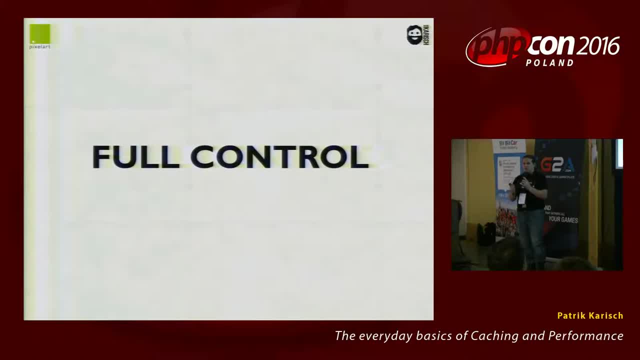 It's your cache, It's your application, And the stakeholders love you. if you can improve the performance of your application, So do caching. First of all, the application cache is key-based. You can imagine every key you want, depending on the cache, how you have a character limit. 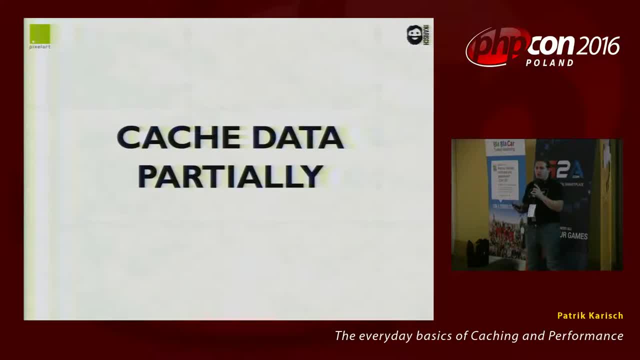 And you can decide if you cache your data partially or you cache your whole page. And you can decide if you cache your data for a single request or for a single instance, like your docker container, like your virtual machine, Or if you have a dockerized application. you have, most of the time, many docker containers. 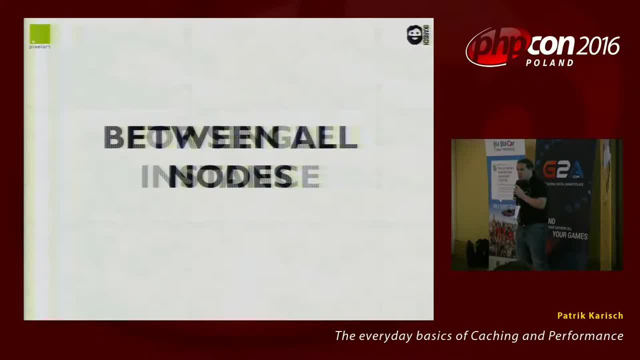 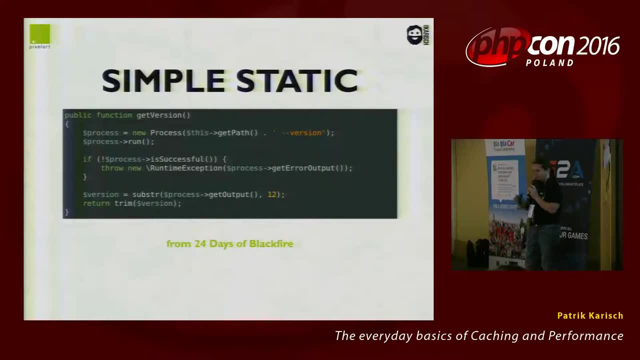 So you may cache on all of them. You may cache on all nodes, on all your docker containers, on all your virtual machines. But let's take a look at a quick example. That's from 24 days of Blackfire. It's a method getVersion, which simply instances the Symfony process component to get the git version. 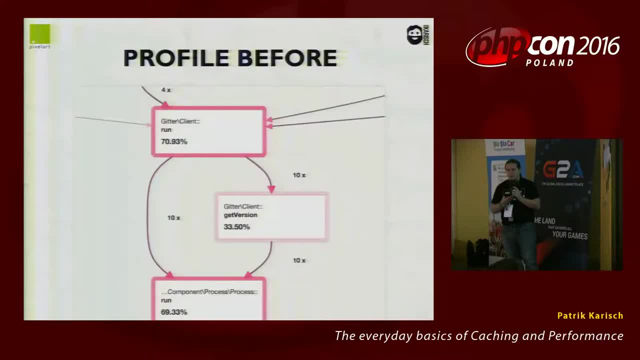 This is a heavy run. If you look at the profile, you always profile your application to know where you have performance suckers. If you have 33.5% of calling this getVersion 10 times, We are calling git minus my version 10 times and it sucks 30% of our application runtime. 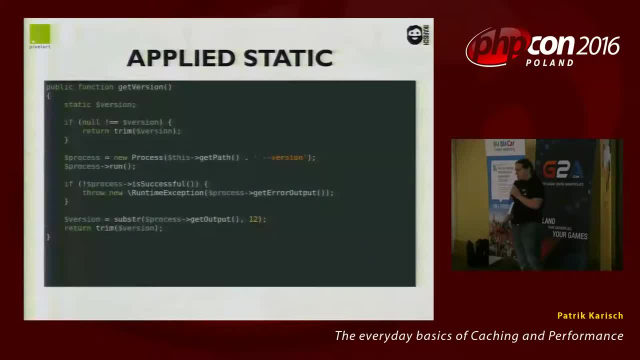 So let's improve this. We could introduce a simple static variable, static dollar version. So we have to test if this variable is null or not. If there is a version saved, we return this version, But if not, we call git minus minus version again. 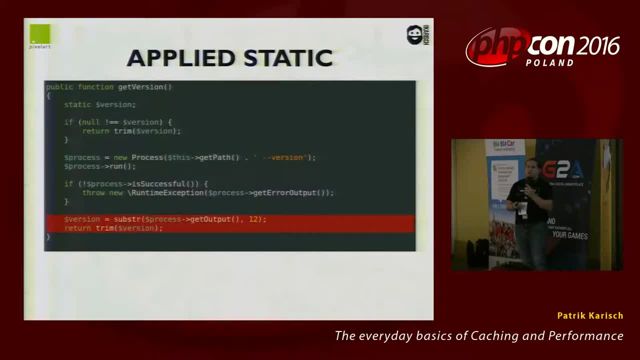 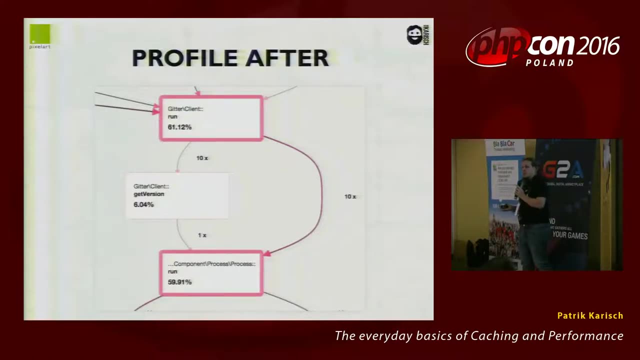 And save it to the version variable and, of course, return it. That's the simplest version of utilizing and cache. But static variable is not the best, Especially it's only for this single request. But let's compare the profile. Now we have only 6% of application runtime to get the git version. 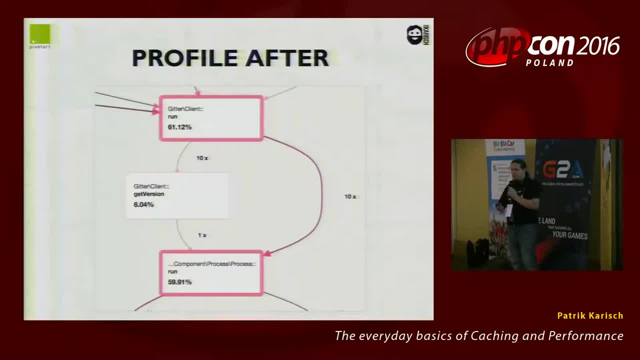 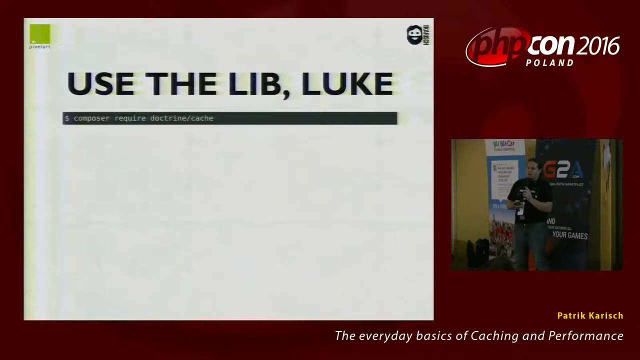 And it's only called once. That's a huge improvement. Okay, But as I said, the static variable is not the way to go, So use a lip look. Please install docring cache Or any of the new psr cache implementations. 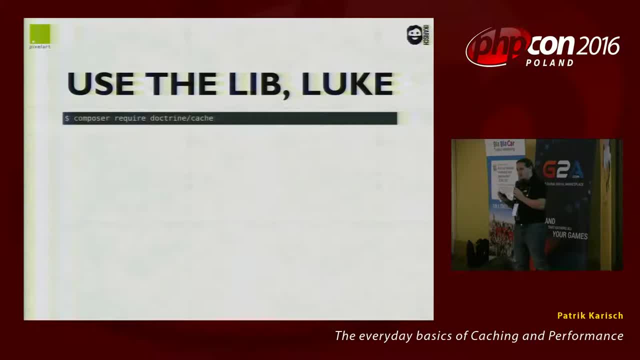 I like docring cache more because the new psr cache implementations have a real cache item interface introduced. That's not nice. I only want to get my data directly from the cache And not with a cache item in between. So install the lip via composer. 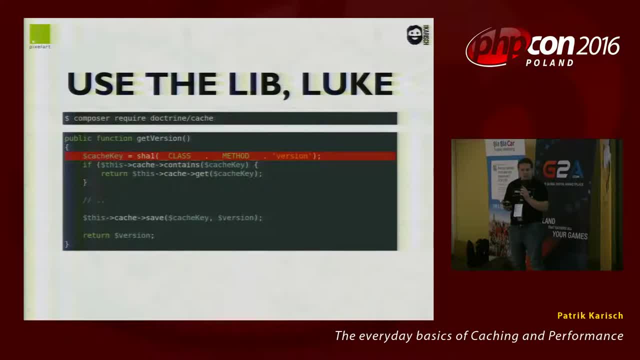 And now imagine a unique cache key. It should be unique, Otherwise you overwrite your cache. In this example it's a shell 1 code of class, method and version. Okay, Then, as seen before, look in the cache if there's an entry. 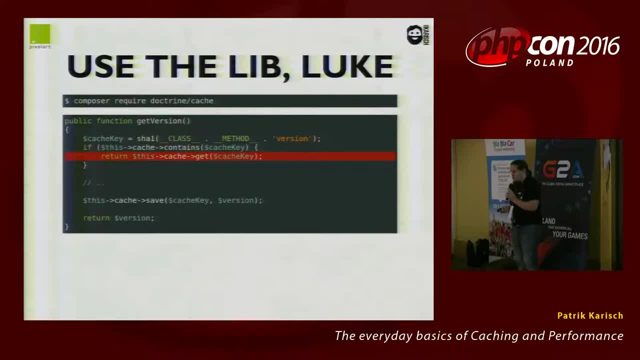 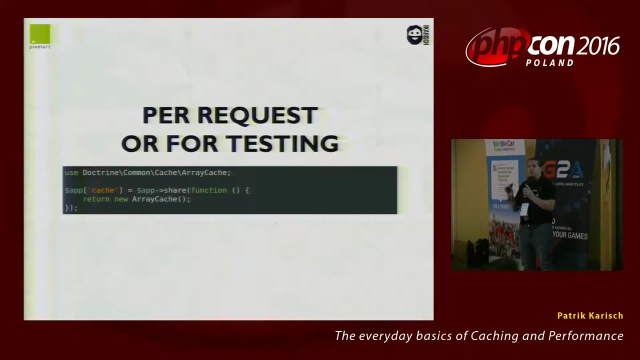 If it's true, get the cache data. Otherwise, compute your version Or whatever, Save it to the cache and return of course. So with docring cache you have different implementations to use. For a single request, or especially for testing, you should use the array cache. 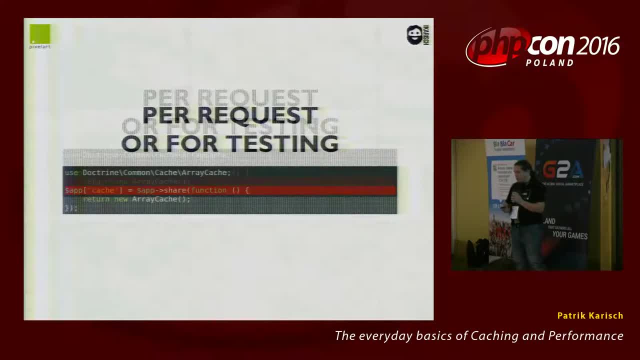 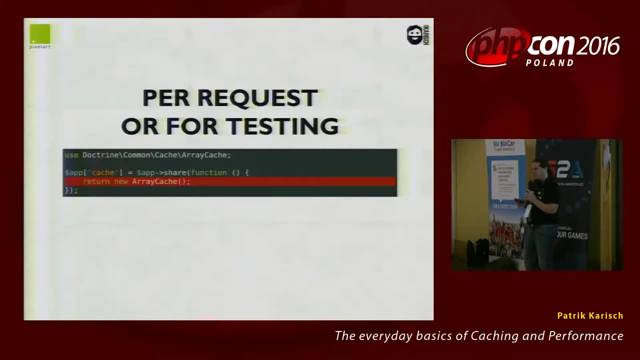 In this example it's silex. I initialize my cache service with a new array cache. Okay, It's for testing. I can't imagine a use case where I want an array cache in a production environment. So use it for testing, of course. 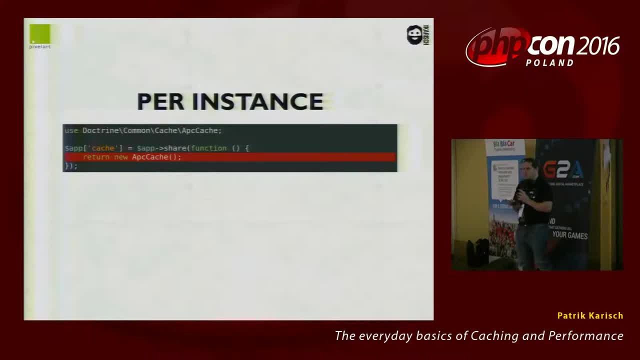 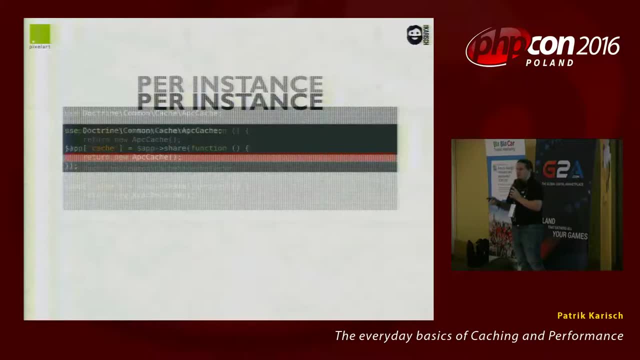 Okay, Per instance, you could use the apc cache, But it's only in your php fbm instance on this specific server. Maybe you want to use xcache. Personally, I have never seen anyone using xcache, But it's there. 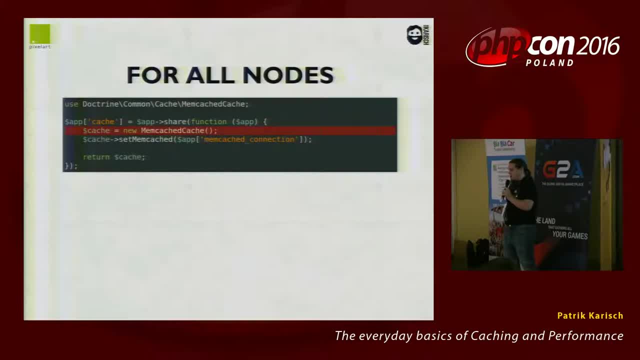 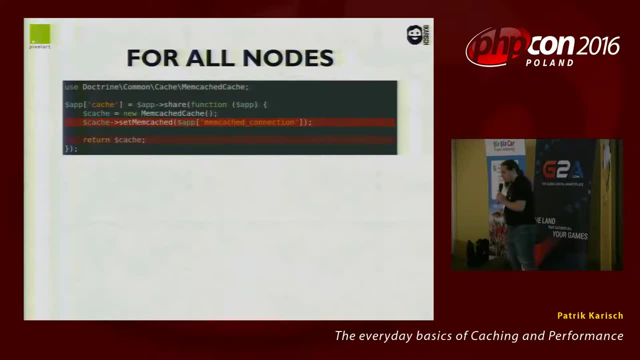 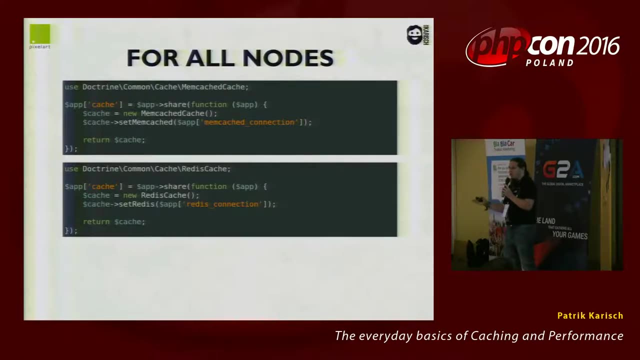 Better cache on all nodes. Whether you want to use memcached- and of course it needs a connection- Construct it on your own, It doesn't matter. Or you want to use redis, It's a philosophy. But if you have a cluster running, cache between all nodes. 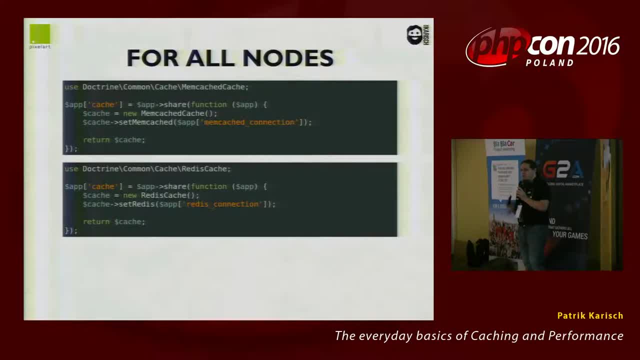 There's only one exception, where you want to cache for a node, For a single node. This is, for example, the git minus minus version. It doesn't matter if you have ansible and so on. You have different versions, maybe on all your servers. 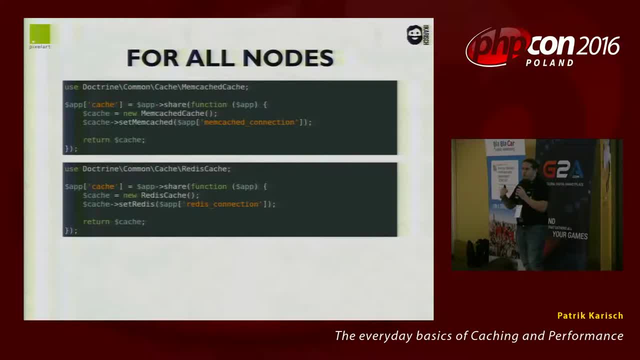 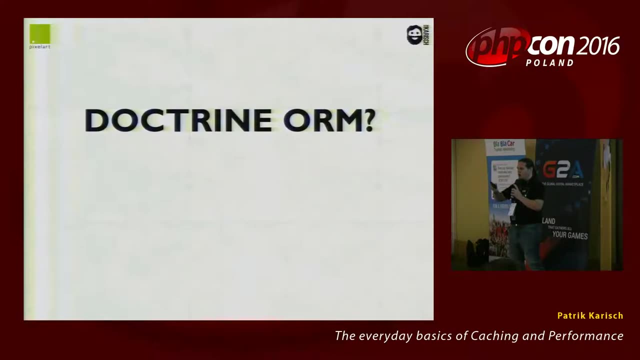 So if you are depending on a value from your machine, cache it only for this machine. Otherwise, all other values should be cached around all your nodes, around all your cluster. Anyone using docreen ORM? Yeah, That's nice. That's what I want to hear. 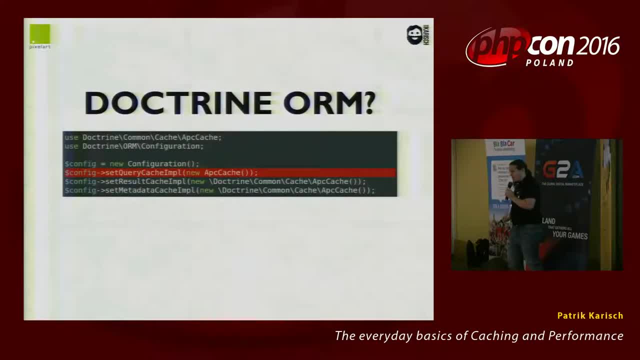 In a production you should configure docreen to use a query cache, to use the result cache and to reuse the metadata cache. You don't want to have docreen ORM running without a cache on production. In this case it's abc. 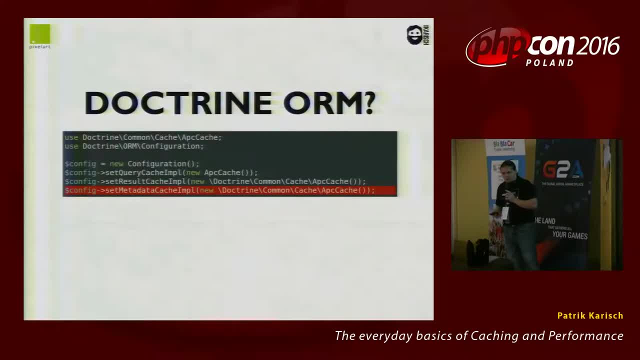 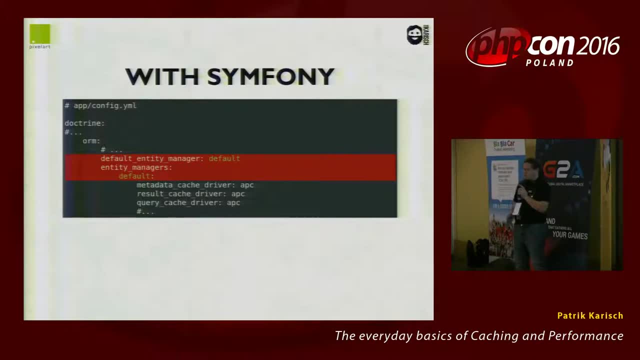 But you should use memcache or redis for a cluster. With symphony it's even easy. Activate it in the config for your entity managers. The same Metadata result and query cache. So the only exception which is not automatically activated in docreen is the result cache. 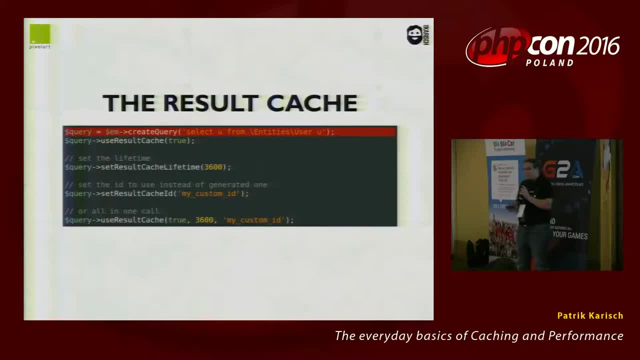 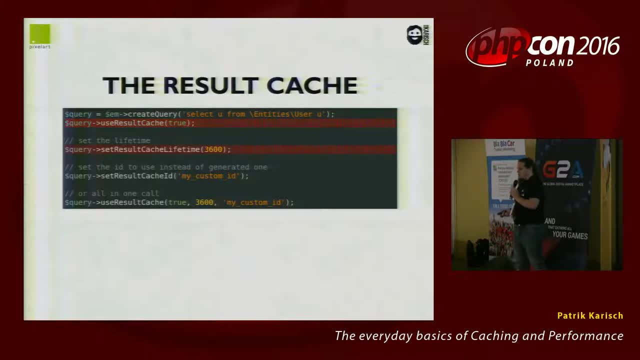 So if you create a query, example, select all users from your database, You can activate the result cache on your query builder on your own. Then you set the result cache lifetime, for example one hour. The users list can be cached one hour. 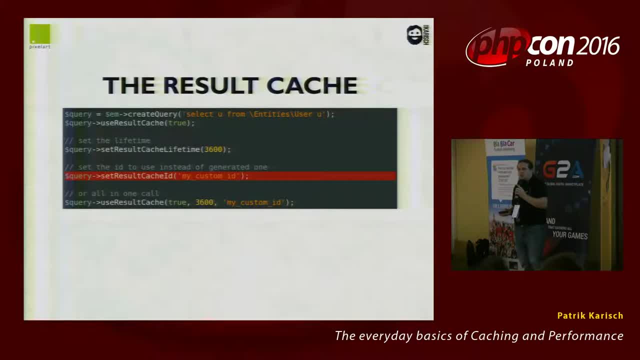 And please set the result cache ID. Otherwise the cache ID is generated automatically and you have a problem to get rid of the cache entry. If you are caching, you always need a strategy to do invalidation of the cache, to delete the cache entry. 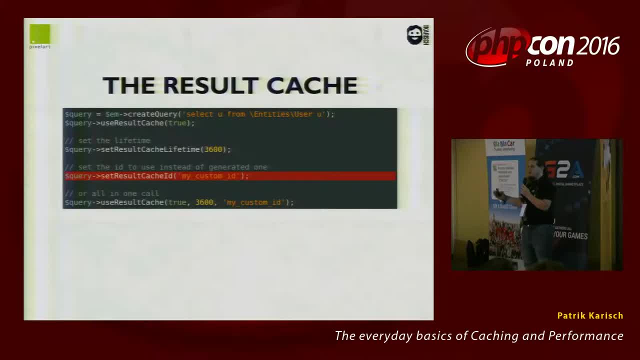 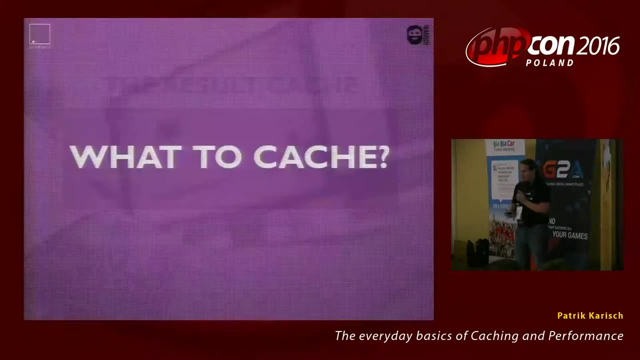 So if you have a backend where you change something of the user, you have to delete this cache entry. So you should use a good result key And, yeah, you can use it all in one line too. So it's specific. You have to know what you want to cache. 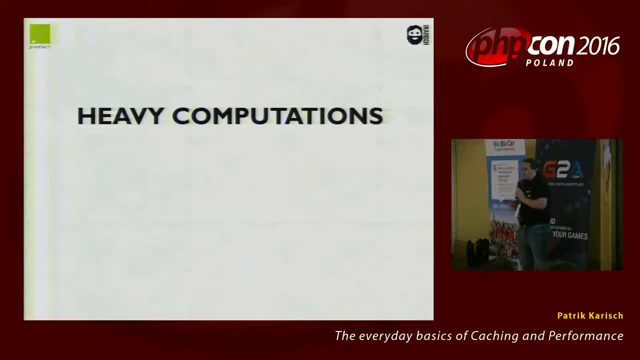 There are heavy computations Like the git minus minus version call seen before, Or everything. Everything you call a binary on your server and so on is a heavy computation. Menu structures, Imaging on CMS with about 500 sites organized in many sub-sites. 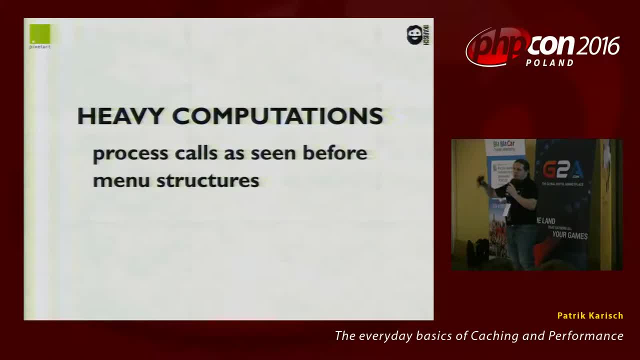 And we had an application where we are generating the menu, getting all sites, Then, for every site, getting the sub-sites and getting the sub-sites and sub-sites and sub-sites. This resulted in like 300 queries. That's not effective. 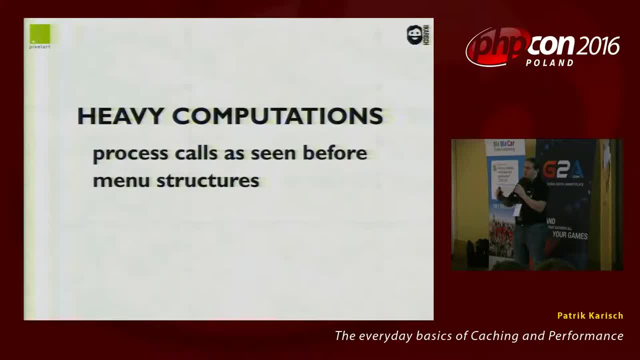 So, simply, we have cached the resulting object tree, The array tree of all sites. And then we had a bad internship, to say, Which has rendered this menu structure into three different HTML output: One output for desktop And we had one output for the tablet. 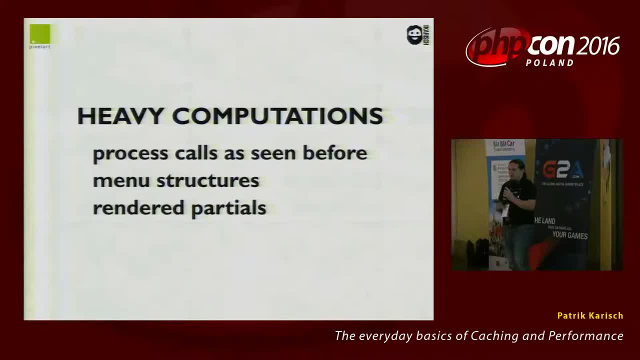 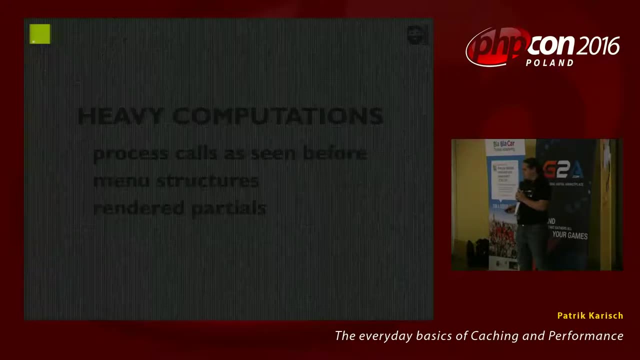 And we had one output for mobile. And that's not fast And simply we have cached those rendered partials. So the first request was sadly slow, But all other requests were really fast Then. Oops, Yeah, Okay, Another thing to cache could be SQL queries. 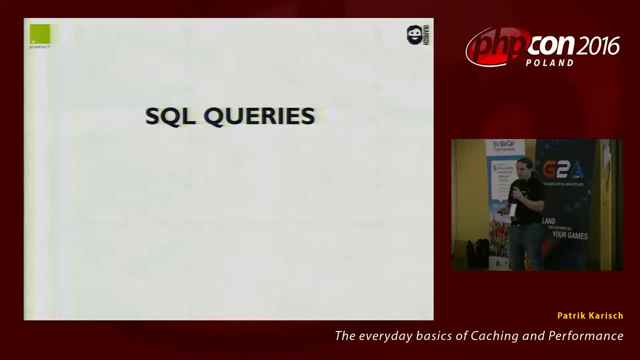 Use the result cache on docrin Or simply use the cache implementation to cache the result of a plain SQL query. Like fat joins, If you're doing a join about over five tables, This will never be fast. It doesn't matter how many indexes. 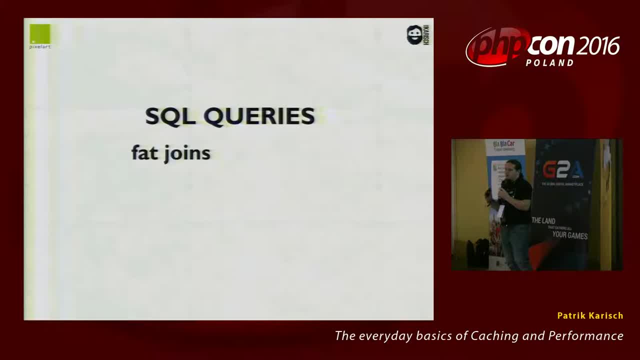 You have A join. about five tables is not fast. You are always creating a temp table And this is slow, So cache the result of those fat joins. Yeah, Slow queries is the same. Maybe you're fetching 100,000 records. 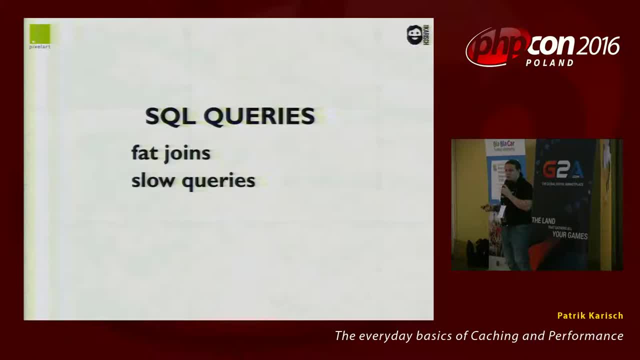 This will not be fast. Cache it too, if it's cache able And often called queries. I have seen applications which have a database table of all countries available. They are great. They are varied in every request. But whoever changes the name of a country expects there's a war and it's conquered by Russia. 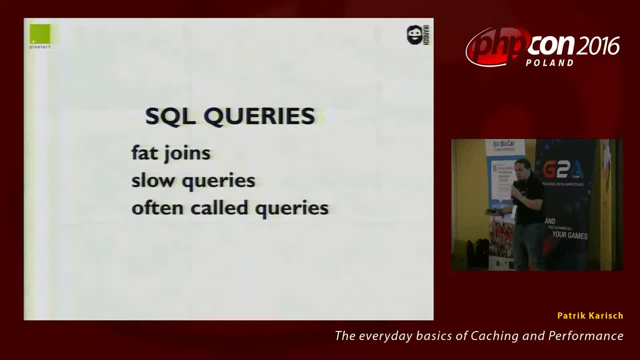 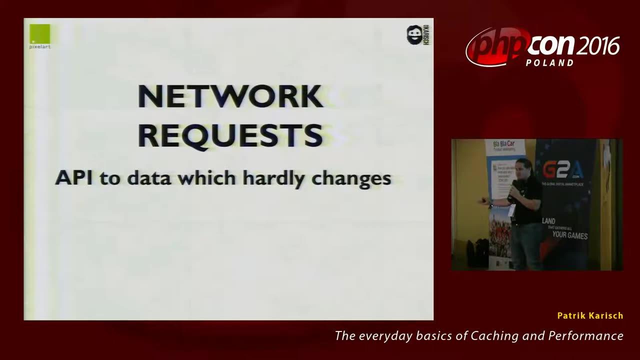 So cache the result of a. get all countries in your cache. Then there are special network requests. What is a special network request to cache? Like an API which data changes, Hardly Like a country API. It's the same Like country table. 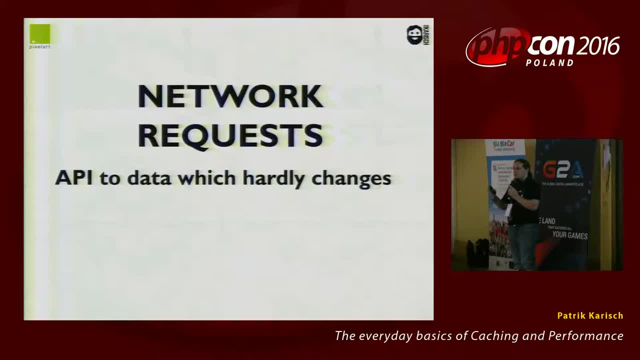 You can cache the result. A good example is a newsletter system like mailchimp or avalanche. They may have an ID to country mapping And you need the IDs. You don't need the IDs on every request to fetch from the API. Cache it. 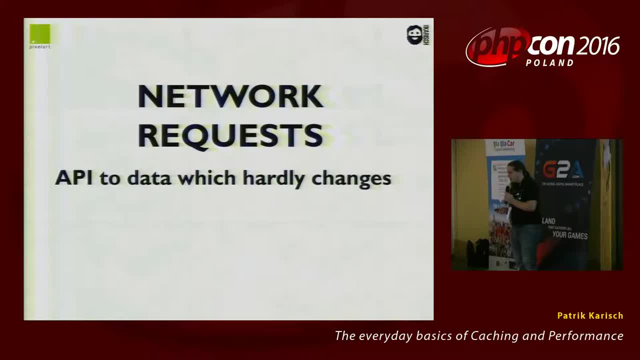 Please cache it. The users will love you if you are fast Or a lower lifetime to data APIs. For example- Sorry, A data API which changes not so fast. You could cache it for 30 seconds or 60 seconds If you have a high traffic application. 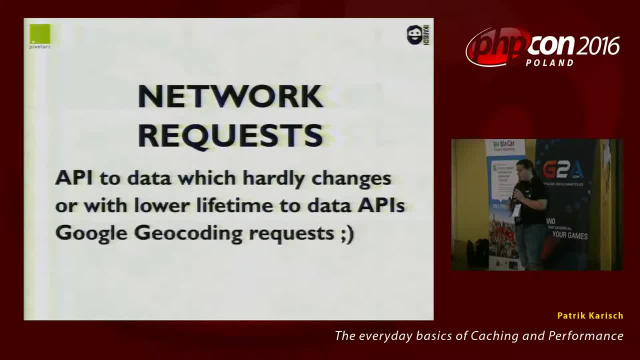 And what you should really cache is Google geocoding requests. They don't like it. if you do live geocoding on every request, on every view of your map, Cache this, Review your geocoding from an address to coordinates or coordinates to an address. 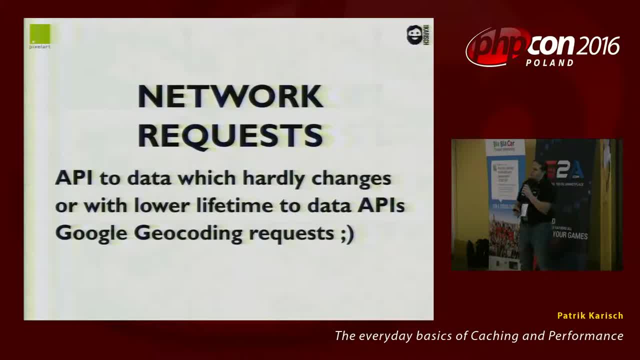 Cache this. Google doesn't like you. Google doesn't like you if you do geocoding on every web request And then there is past config, like yaml xml annotations. You don't want to pass it on every request, It's the same. 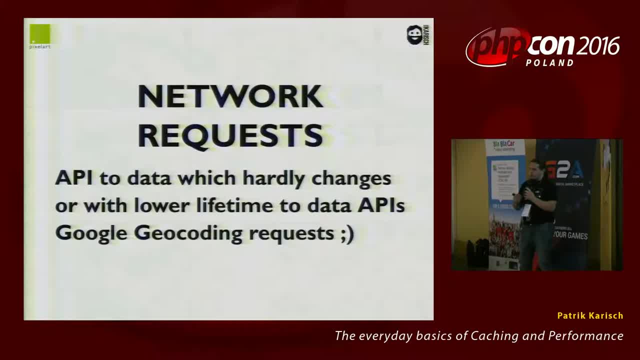 Compile this stuff to php, Even your template, just like twig does Or like the symphony di container does. It constructs a big php file with all instantiation of your services, And that's nice and fast. The symphony routing is also fast. 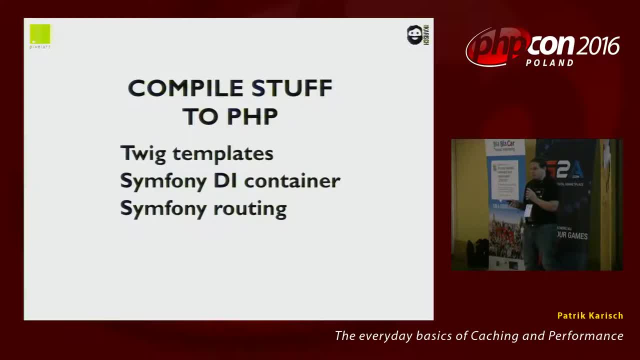 They even removed the apache hate, the access dumper, Because they say the symphony routing in php is even faster than apache rewrite rules And symphony translations from yaml, from xlib files, is also cached to plain php files with an array of all translations. 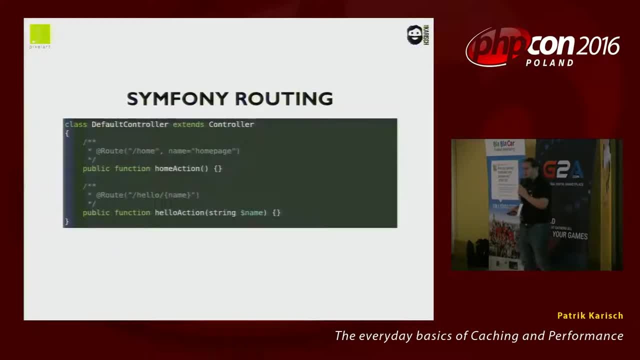 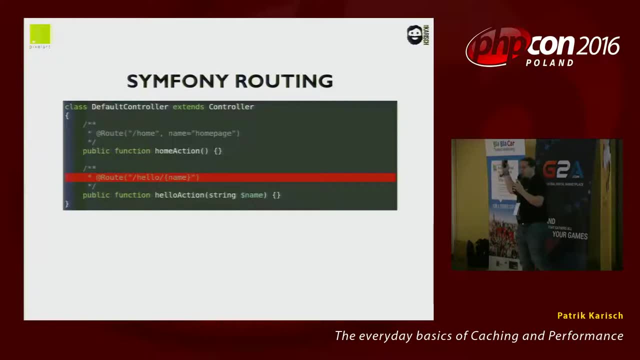 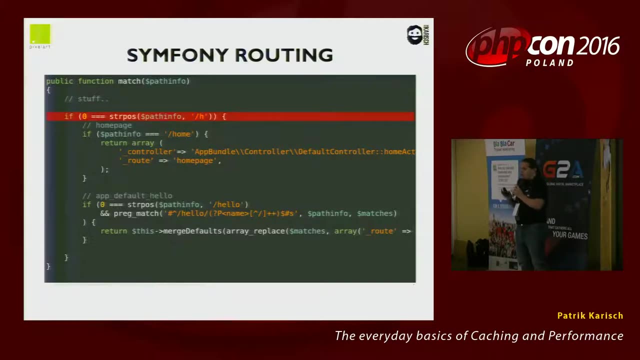 For example, let's take a look at this routing. We have a home route, slash home, We call it home page, Okay. And we have a route slash hello, slash some name, And this is the cached routing matcher. At first we can look if the route begins with slash h. 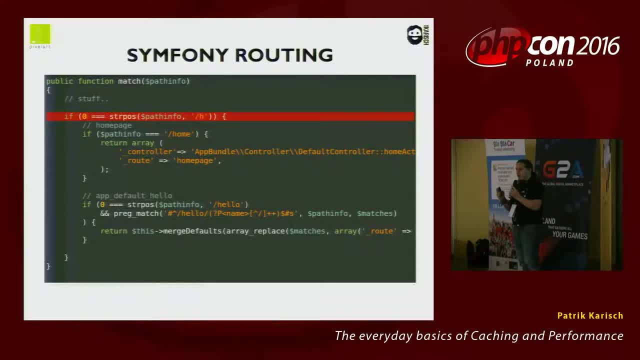 If it's not, we skip a whole if block. If you have many routes starting with h, we are skipping, for example, 500 routes, And this is fast. Then we can look: Is the route slash home directly? If it's so, we return all the controller and route attributes. 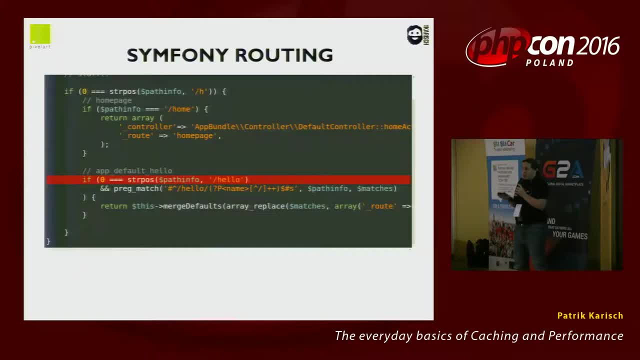 If not, we go further. check if the route begins with slash, hello. If it's so, we can do a break match to extract the name and so on. And this is really fast. So if you have some configs, cache them. 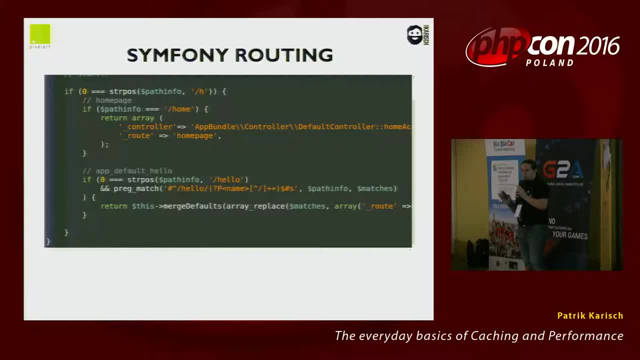 Have you any questions to php compiling? It's not easy to do this. The symphony router is a real complex class, For example, If you have ever time to analyze this- But it brings you real performance. So let's recap this. 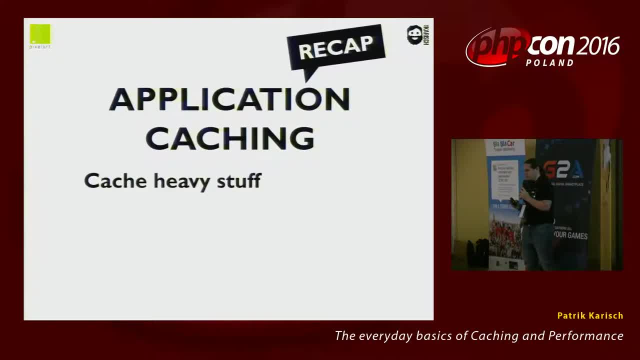 You should really cache all your heavy stuff And at least have an invalidation strategy. As said, if you do caching you have to delete it. I mean, if your lifetime of the cache is 30 seconds, it doesn't matter. 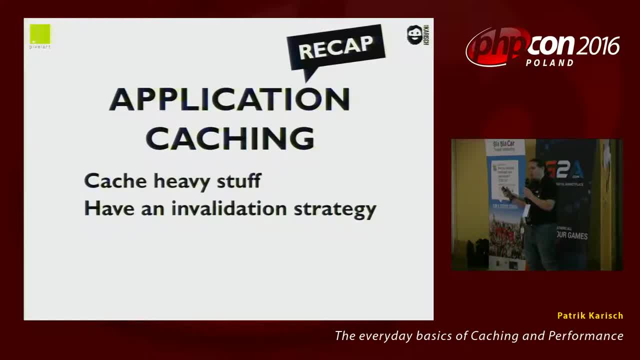 But if you cache some data for one hour or for one minute, for one hour or for one day and you have to edit it and you have full control in your application, not like in the browser cache, then you can delete it. 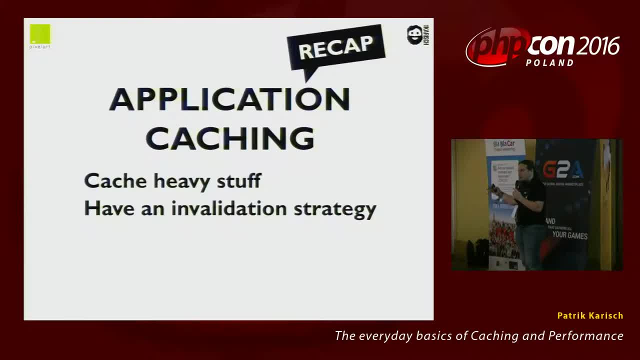 The editor of your cms edits stuff like the page in a menu structure and the menu structure is deleted from the cache And on the next request it's generated again And use a library. Please use a library If you don't use a library to do caching. 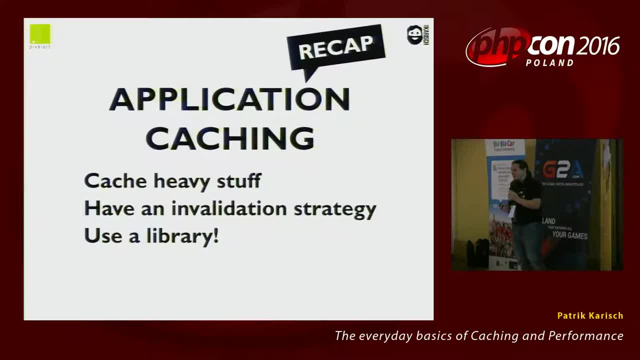 will come to your house on the roundhouse, kick your door and destroy all your data. Okay, And compile some configs to php. Really, You don't like to pass your damn yaml config every request And profile your application, Please profile. 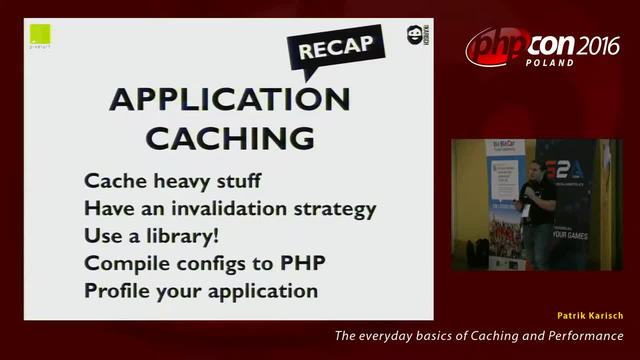 Nowadays, with Blackfire or Tideways, you have no excuse to not profile your application And look where you have performance problems. So now everyone knows how you can do this. Everyone knows how you can improve the performance with caching in your application. 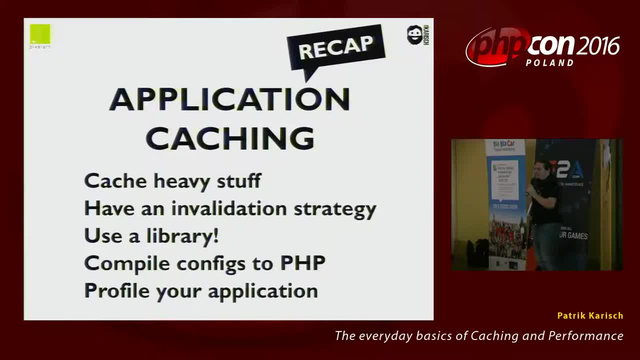 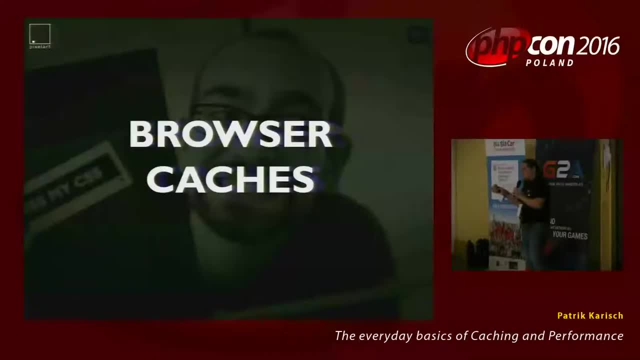 Looks not so lucky, but I hope so. On the other side we have application caches. We have our gateway cache, proxy cache, and then we have the browser cache, And browser caching can be fun, but it's not really fun. 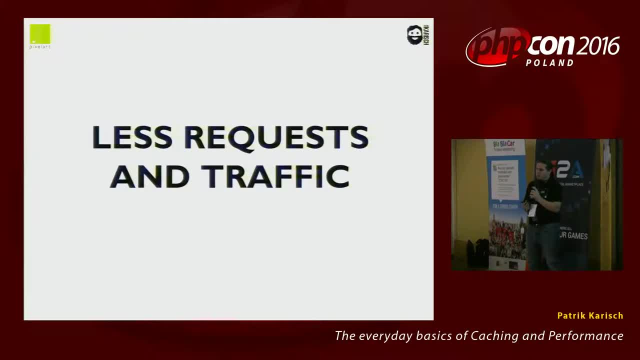 The pro of browser caching is you have less requests and less traffic. If you're in a cloud and have a high-performing website, it means of user traffic. You pay terabytes of traffic. If you can improve this with browser caching, you can save thousands of dollars. 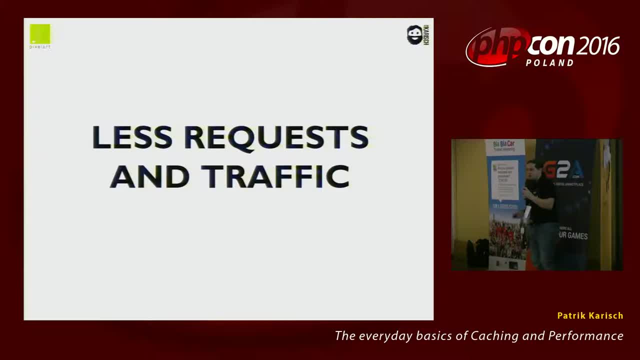 or 10,000 of zloty, And the downside it's client side. It's only in the browser, of course, and you have no control of it, which means you can't say to the hey browser, please delete this entry. 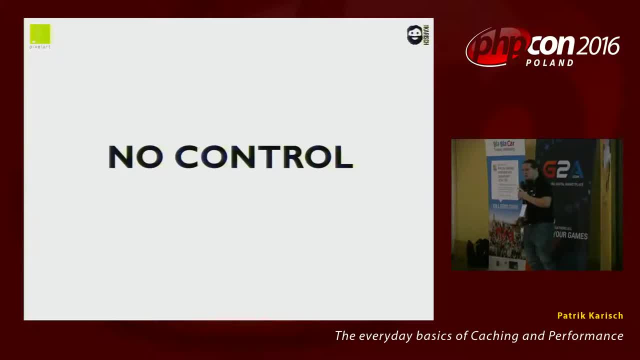 I want to send you a new one. Let's do this. There's one exception with changing the url in the linked html file. Like cache busting, we do every time with javascript and css sources, But basically the cache in the browser is url-based. 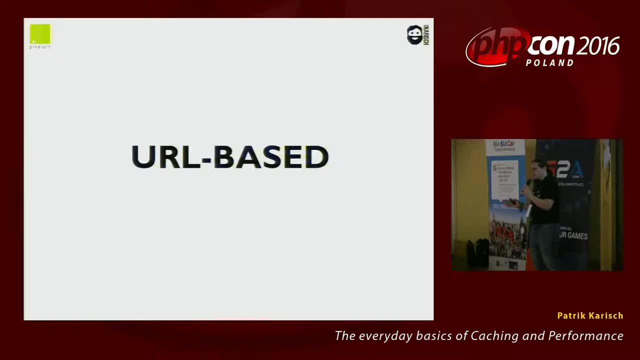 One url is one cache entry. Of course. I said with cache busting you change the url, you get a new cache entry. You have no invalidation. I said you can't delete some stuff in the browser's cache And it's a simple lifetime. 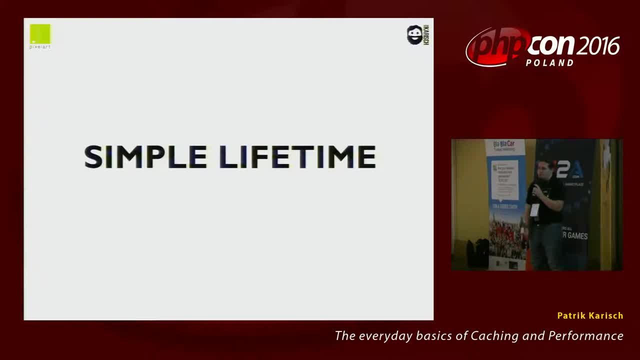 You can define, say the browser: hey, cache my site for one hour. Or you can say the browser: if you have the site, please ask me if you can use this in the cache or not, Or you can use both. You can say the browser to cache it for one hour. 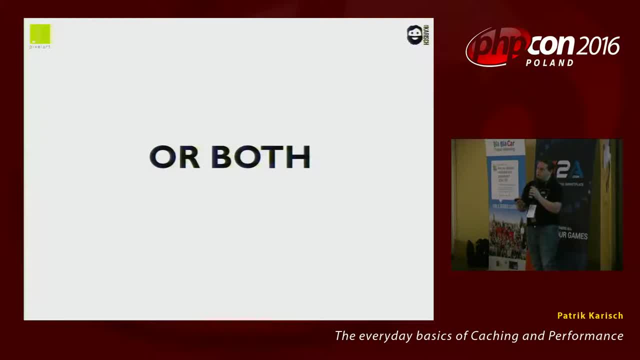 and then, if the one hour is over, the browser asks you if it's fresh or not. So let's take a look at expiration. That's the simple cache control header you can send with a max age of half an hour and a shared max age of ten minutes. 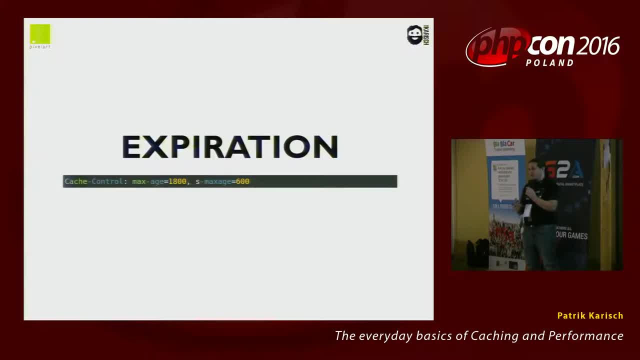 And this is not a typo, It's written as it is. Max age has the minus between max and age, And the shared max age has the minus between the s and max age. Standards- Real cool standards. So the best is to use a library. 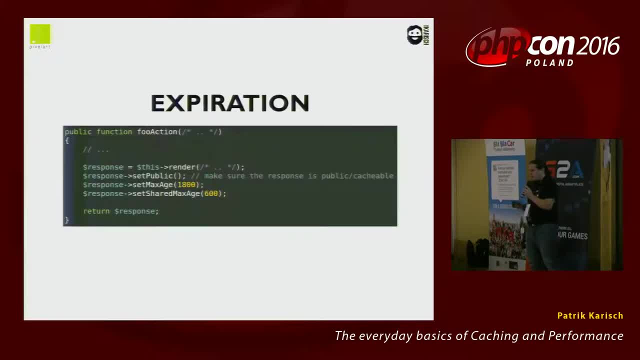 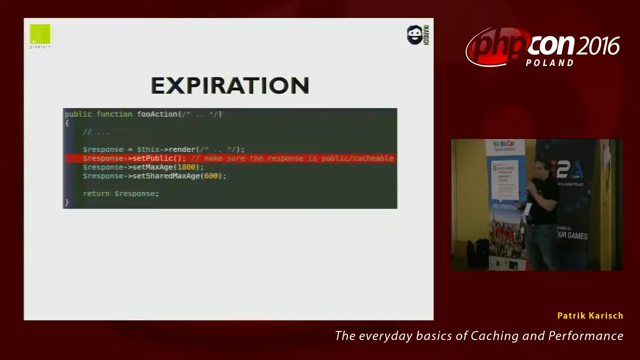 Or if you're using symphony, you have it already. At least use the symphony http foundation or any of the new PSR 7 middle http message implementations. In this case, we simply render. whatever we render, We set the response to public. 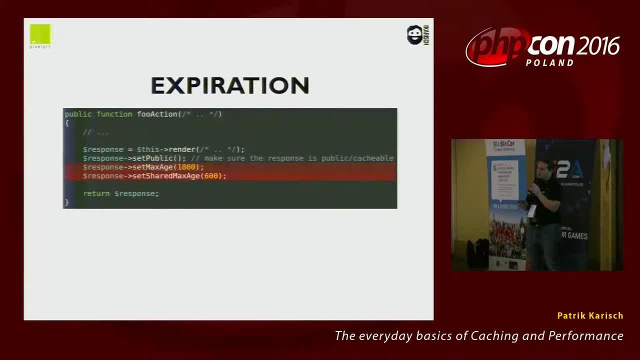 We set the max age of half an hour And we set the shared max age for proxies. The shared max age is used for proxies and gateway caches, not for the browser- to ten minutes And that's it. So we say to the browser: cache this page half an hour. 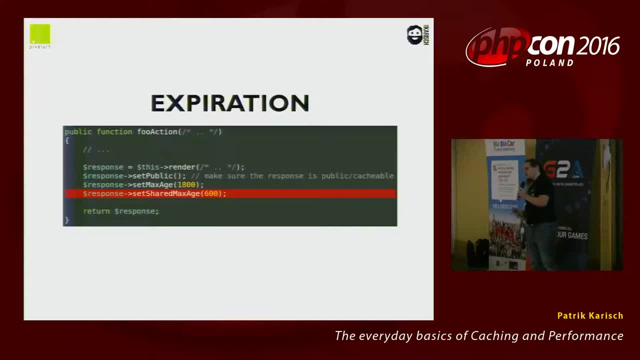 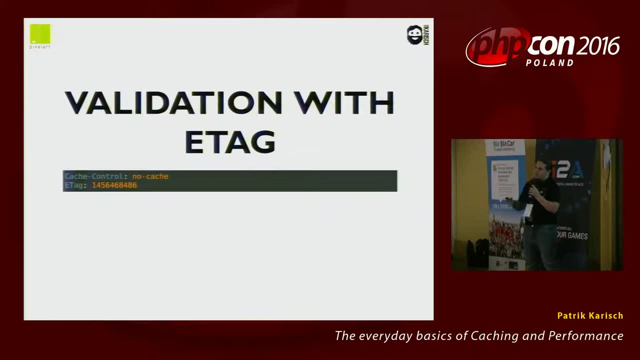 and then come back to me. But you could do the same with validation, which is not caching in the browser, but instructing the browser to ask you: is it fresh, is it fresh, is it fresh on every request? ETag is something like an entity tag. 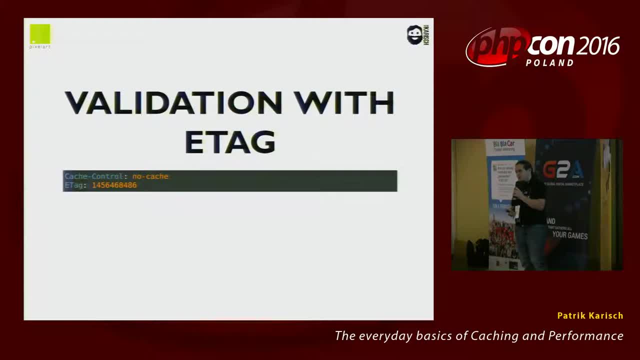 It can be anything. I show one hash of your entity, a time stamp, a per Customized string, whatever, It doesn't matter. You simply send cache control, no cache and an ETag. And if the user visits the site again, 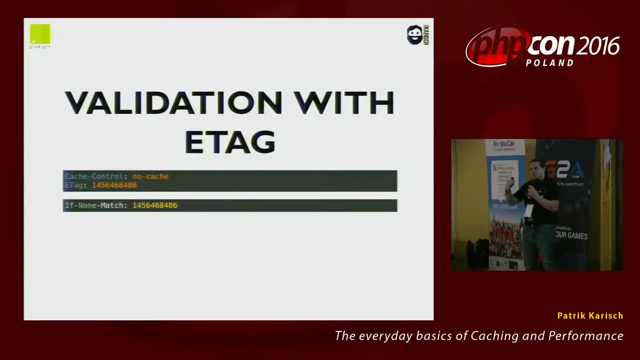 the browser asks you if none match and the same ETag you have sent before And if it's really fresh so you don't have changed the site, you can say 304, not modified, And the browser reuses the page he has in its cache. 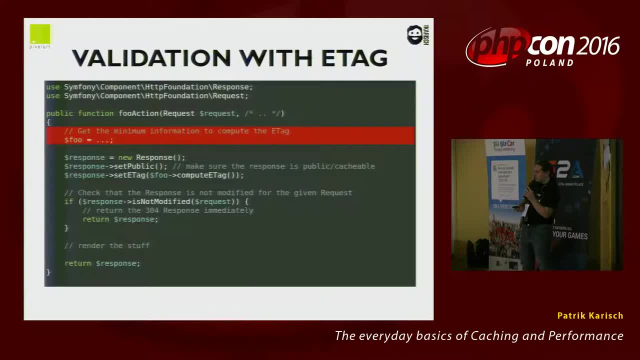 This is Another Symfony example: Render your. In this case you need to get your entity or whatever to compute your ETag. You don't need to render the page, but you need the entity to compare if it's fresh or not. 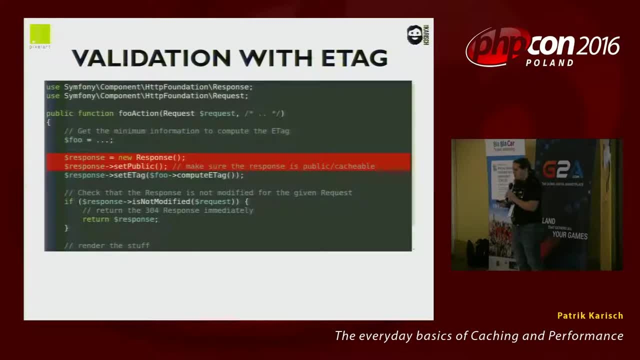 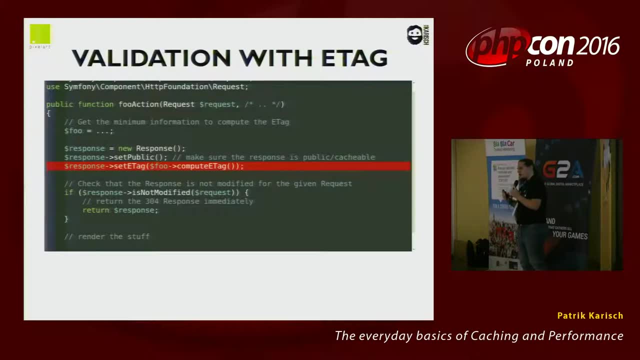 Then you create a new response, set it to public, as you should, and here you set the ETag. Please use compute ETag or a similar function on your entities or whatever you're using. Don't do the computation directing the controller. 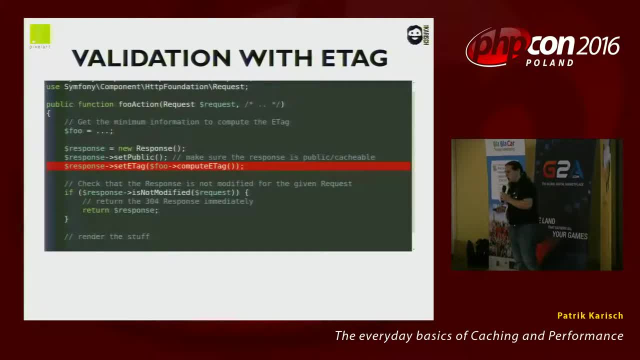 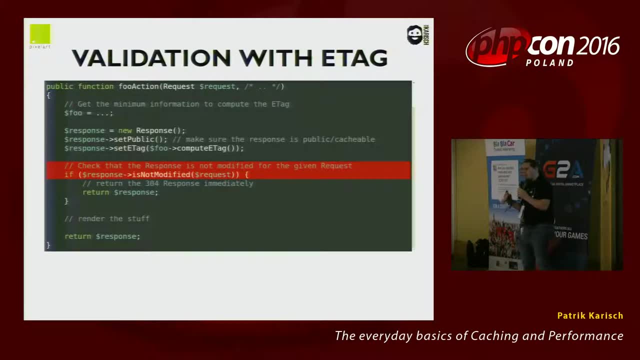 And after you have set the ETag to response, you can ask the response to compare with the request, with the if none match header, if it's modified or not, and simply return the response. In this case, Symfony already sets the correct status code. 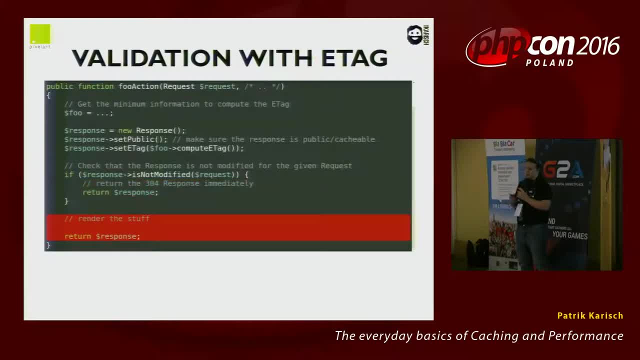 And if it's not, If it's modified, it's false and you simply render the stuff the rest of the page and output it. Okay, If you don't have some data to compute the ETag or it's too heavy to compute the ETag. 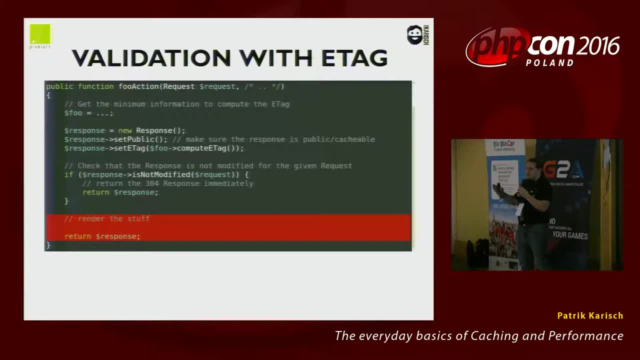 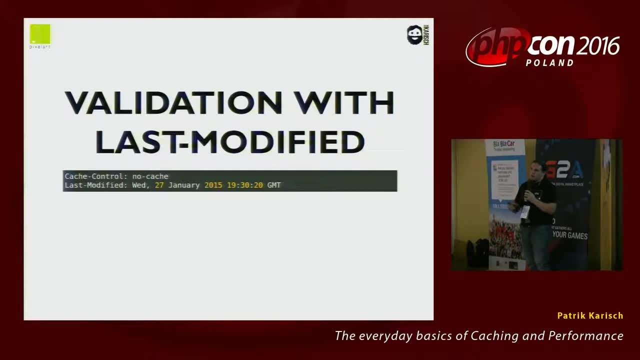 because your model or your entity is so complex. you may use the last modified header. You simply send the last modified header with a perfect, standard-sized date time. That's the expected format, No ISO date. It's really weird. And if the user visits the site again? 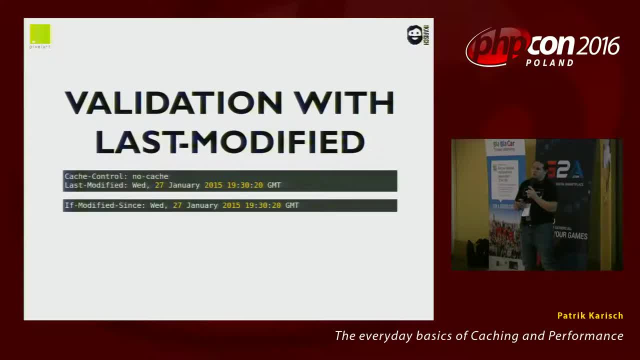 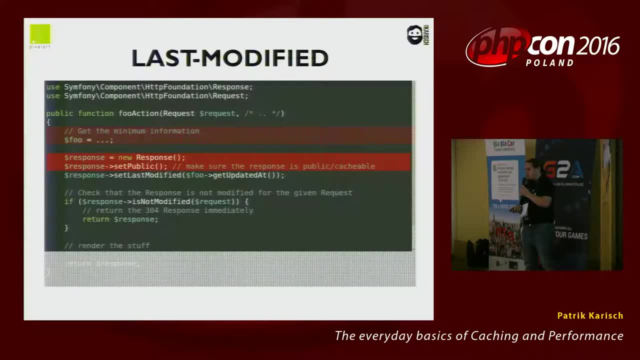 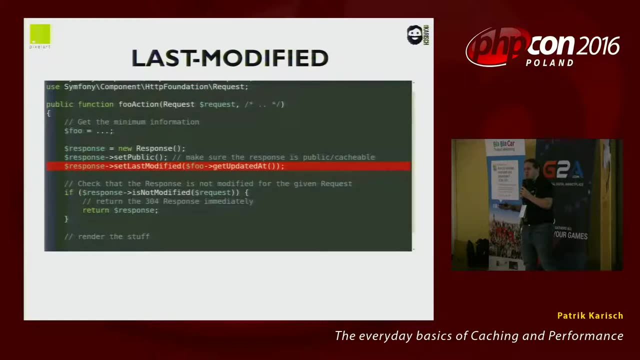 it asks you if modified since header instead of if none match. So if it's match, returns 304, not modified. The same code, with the only difference you set last modified with, for example: get updated at if your entities have a good timestamp error behavior. 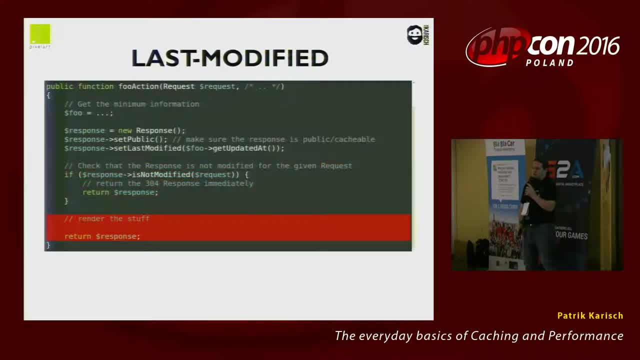 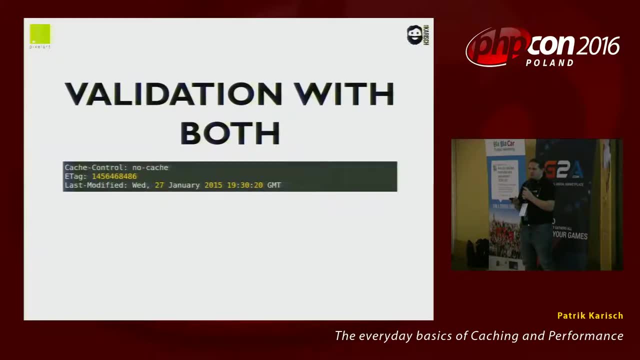 Test it, return it and render the stuff if it's modified. You could do both. I can image in a scenario where I want to use both the ETag and the last modified, but you can't do it, So you should know it. you can do it. 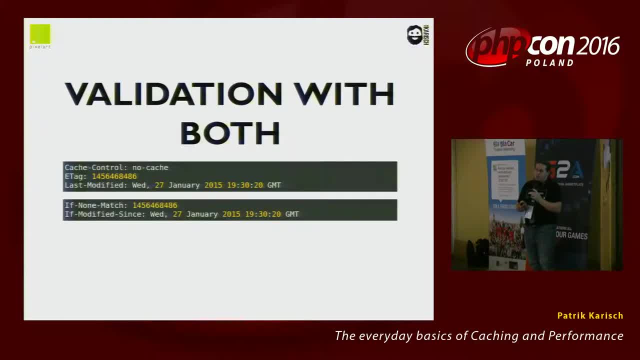 In this case, the browser asks you if none match and if last modified, And only if both are correct. if both match, you can say it's not modified. Otherwise, if the ETag differs or the last modified differs, you should return the content. 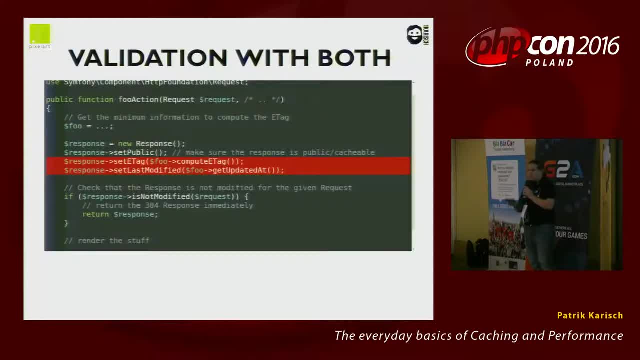 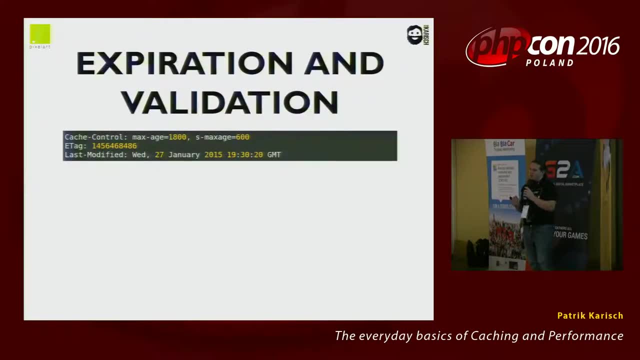 Same example: get your data set ETag and set the last modified, Test it and return And you can combine all three together. You can send a max age and do validation. In this case it can get a bit complicated, but only if the max age is reached in the browser. 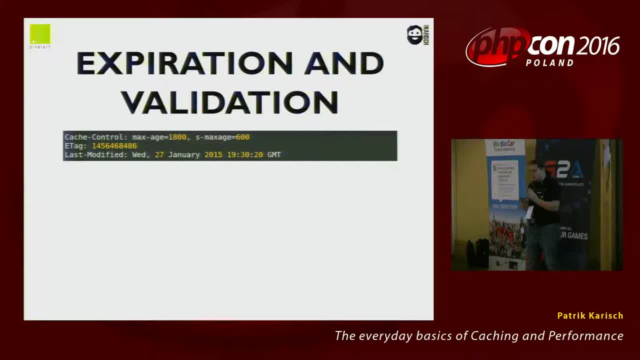 So the entry is stale. the half an hour is over. in our example, The browser asks our server with the same, if none match, if last modified headers, if he can reuse the cache or not, And in this case, if you're returning the not modified 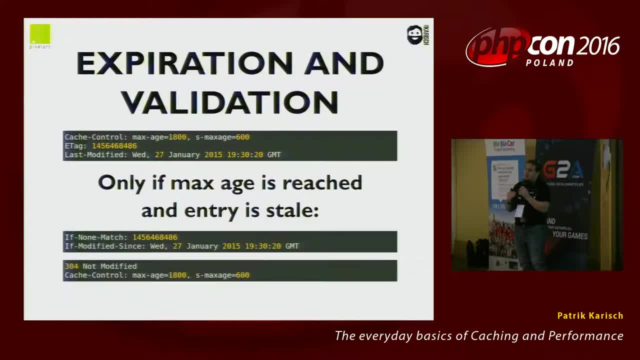 you should return also the cache control header with max age again, So the browser caches your page a half an hour again. If you forget the cache control header with max age, you don't have validation, only validation again, No caching lifetime. So that's really important to don't forget. 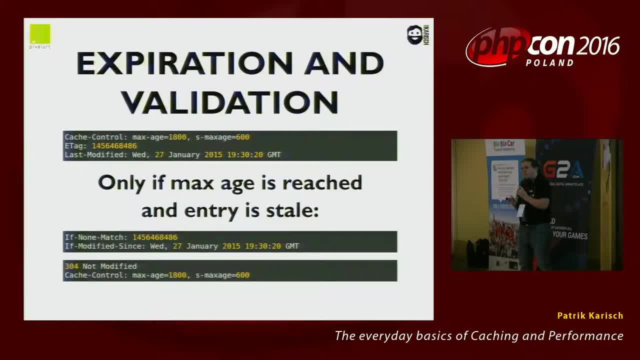 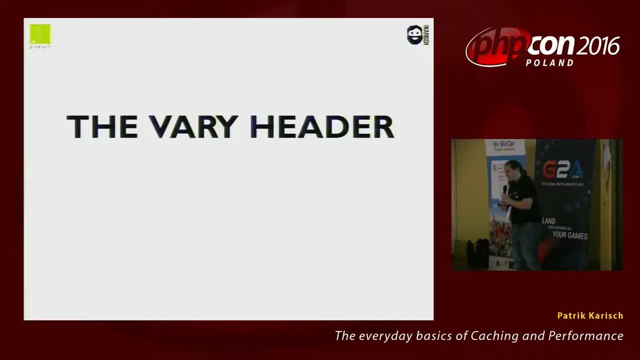 the cache control max age header. if you do lifetime and validation together And then there's a special header, the vari header, It looks simply like vari accept. So you are instructing the browser to get great separate cache entries depending on the content of the request header. 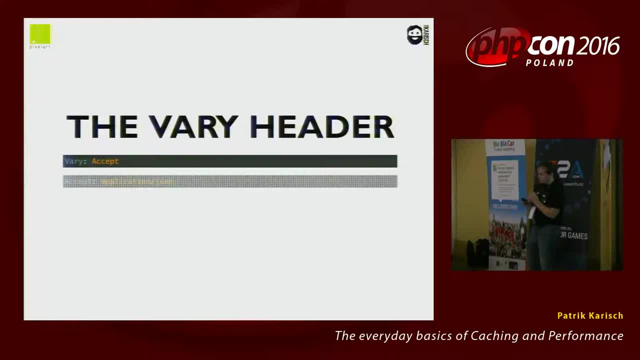 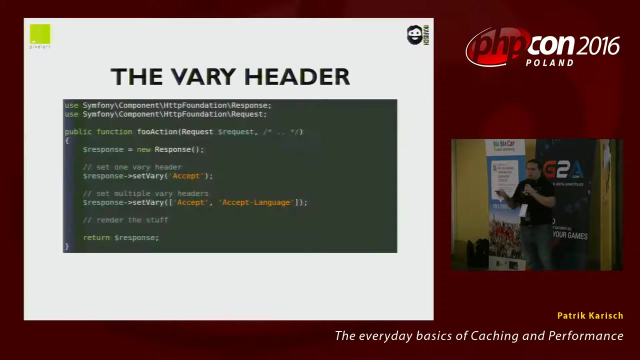 except in this case For an API example. the browser could say accept application JSON. or he could say you want application XML And if you return vari accept, the browser will create separate entries depending on what content type it get requested. Sorry, It's the same with a symphony HTTP foundation. 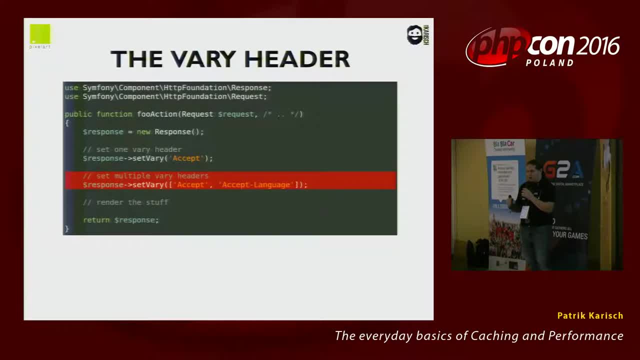 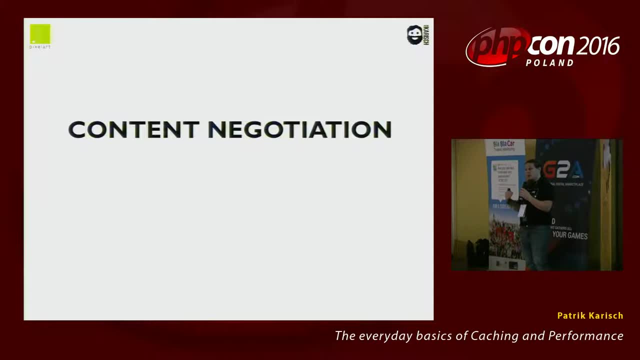 Simply set vari on the response or multiple vari's. Where is this useful? For example, for content negotation. you want cache pages where you have content negotation, like the accept header which negotates you the content type of the page Or you're using accept language. 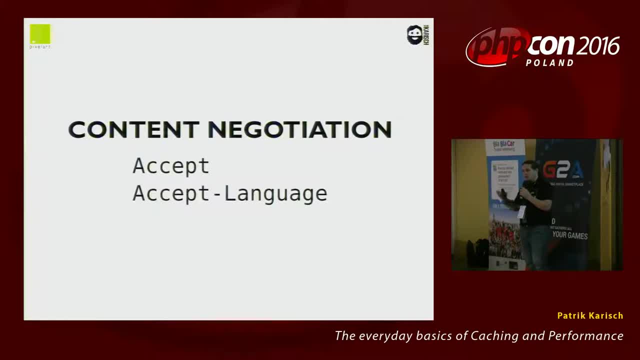 to return different translated pages on the same URI, On the SEO view for Google et cetera. you shouldn't return different translations on the same URI. So these are not really headers to vari on. The only header you can vari on on a cache. 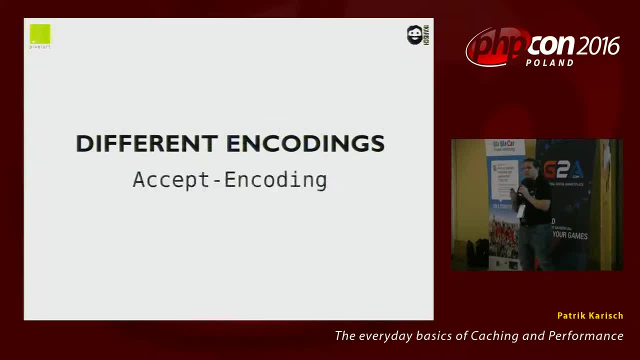 is really for different encodings: the accept encoding header. Accept encoding is for compressing. like gzip or deflate, Browser may compress your, may your page wanted to compress or not, And if you don't send the correct vari header you can have gibberish in your browser. 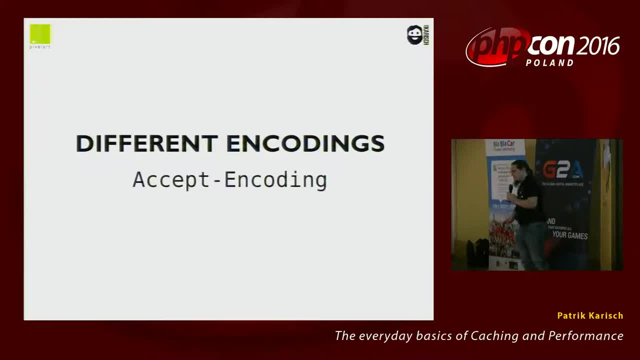 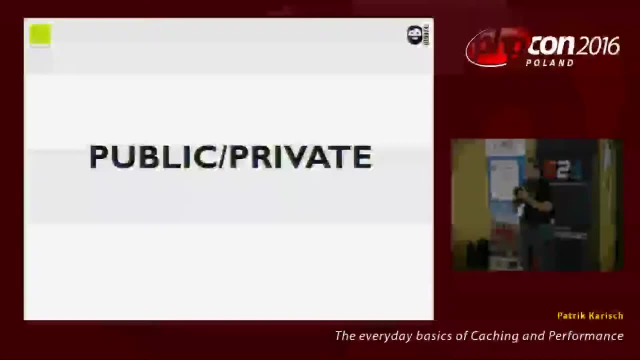 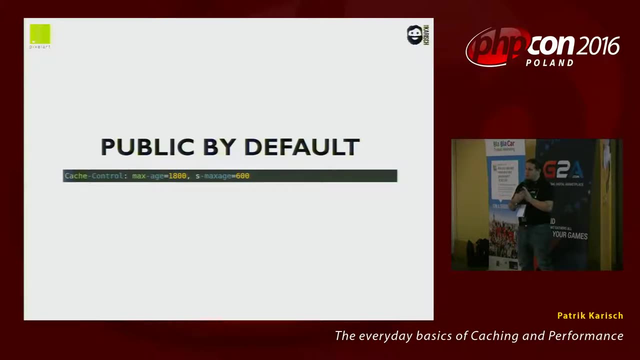 and your users hate you if they say gibberish And special things to take care of while you do browser caching. It's the public-private thingy. By default the cache control header says it's public, even if you don't write public in the control header. 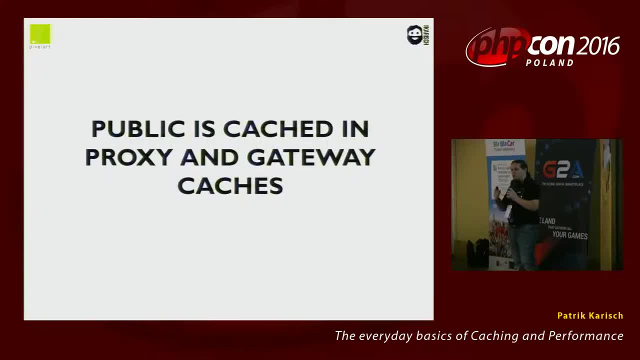 Public means it's cached by all proxy caches and gateway caches in between the connection to your server and the browser. Don't cache user-specific stuff like graded card data et cetera, in a proxy cache. That's not cool. So you say the browser, it's private. 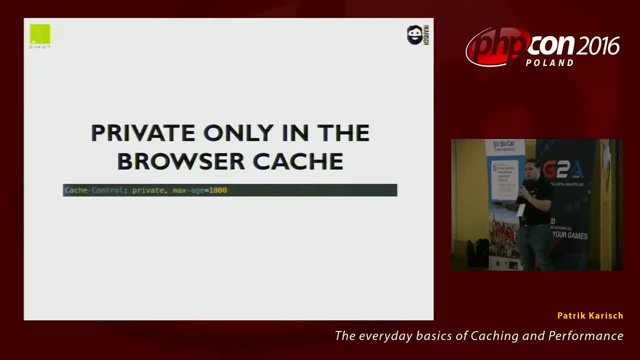 Private means no proxy and no gateway cache in between is allowed to cache it. Only the browser is allowed to cache it. And the lifetime: You should really get a plan which page should get which lifetime. It can be complicated but we will see in a use case later. 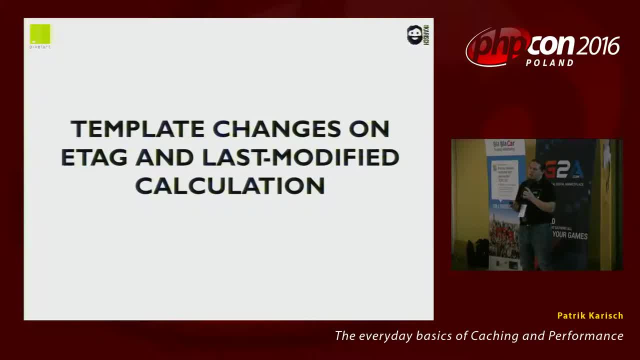 And template changes are not reflected in your e-tag or last modified calculations. So if you have a template bug, like a wrong table or a wrong div set, and you change it, fix it, deploy it. the user will not recognize it until the lifetime of his cache entry is over. 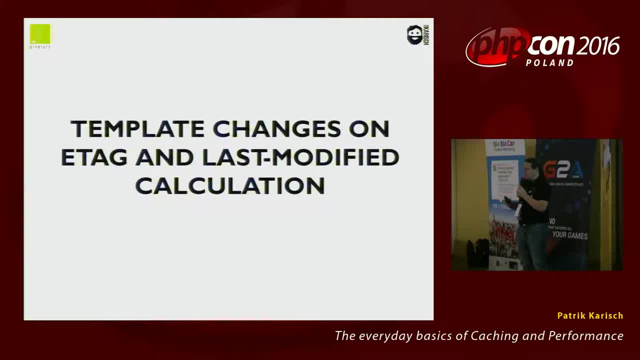 or if you're only using validation, But, as I said, it's not reflected on the e-tag unless modified. So if the user validates his site, the browser with, if none match or if not modified since, then it's not reflected. 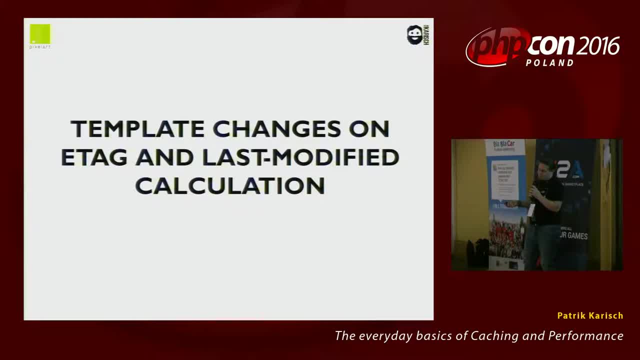 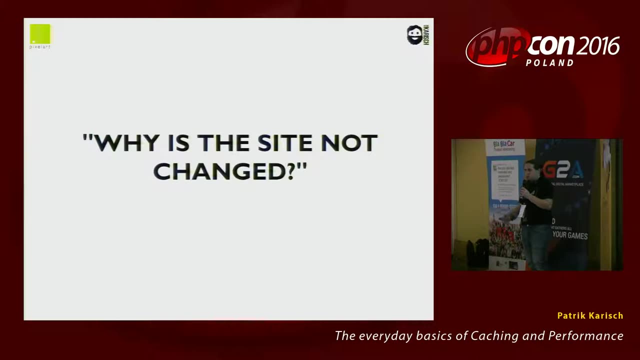 and the user has the old page, the broken page, for it, if you are unlucky. And then there's the annoying one- the customer, Customers are always a problem Like: why is the site not changed? We have cached it. It's for performance reason. 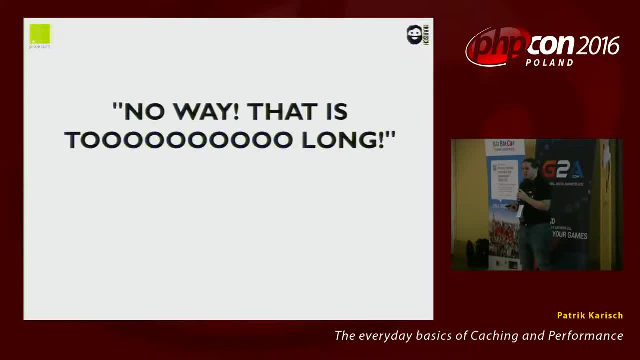 Or no way. that's too long. In the project. we have a simple block with a new post per month. one post per month, And it's too long for the customer? Yeah, Fuck it, And then I need the change immediately. 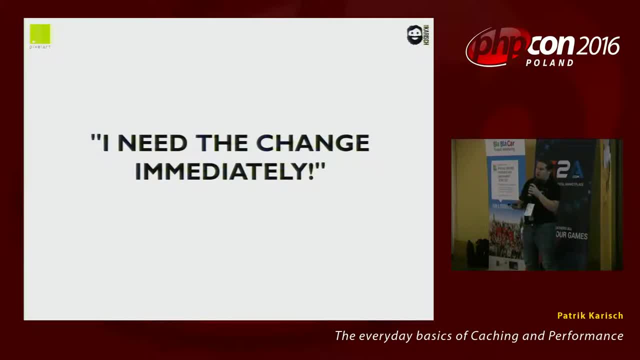 All the stuff they wanted to change. want to see it immediately? Okay, press F5 and you see the change. Your user's not, but that doesn't matter. So you may have problems with the customer if you do too long. browser caching. 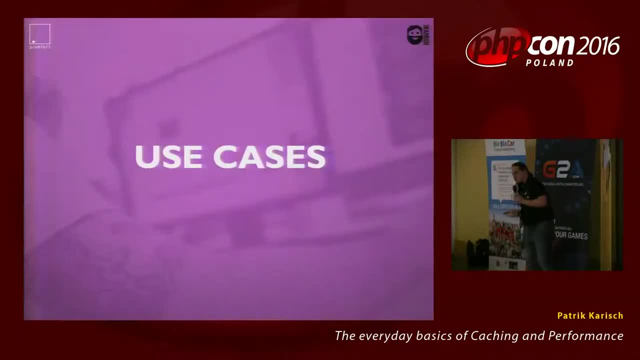 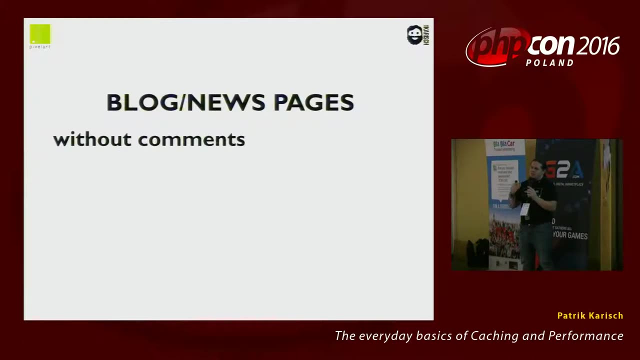 Some use cases. for you. I say it's a block news page, but only if you don't have a commenting system on it. If you are doing comments in your application, it's not good to cache. Maybe use this cast, which is lazy loaded. 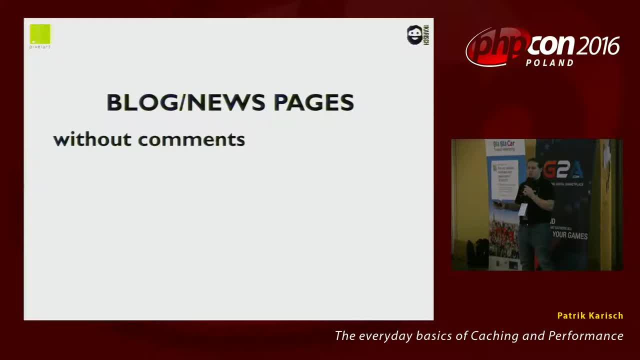 via AJAX or JavaScript, then you can cache the block or news page again. And please use an incrementing lifetime If you are publishing a new post and it gets rushed by 10,000 of users and you have a 10,000 users. 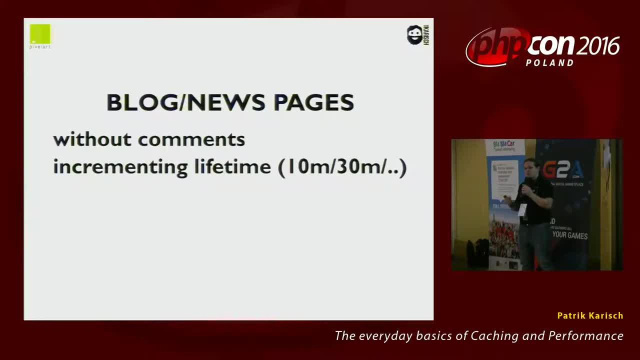 and you have a technical error, then you can't fix it for the users if you cache it for one day. So if you are publishing a new post, cache it for one minute for the first few days, Then after three days cache it, for example, for 10 minutes. 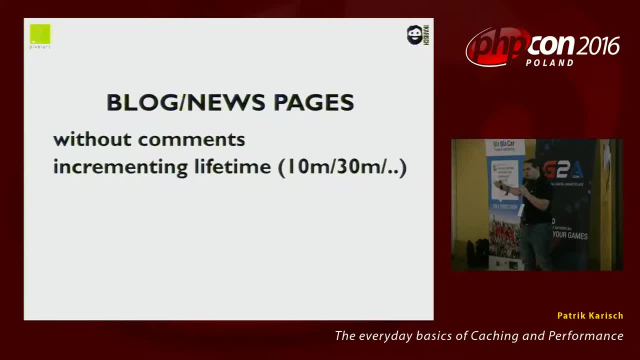 and so on. After the lifetime of your blog post, increase the cache lifetime So you don't have a problem fixing typos or technical errors, Because it's not nice if you write in the comments. now, I fixed it. please look again. 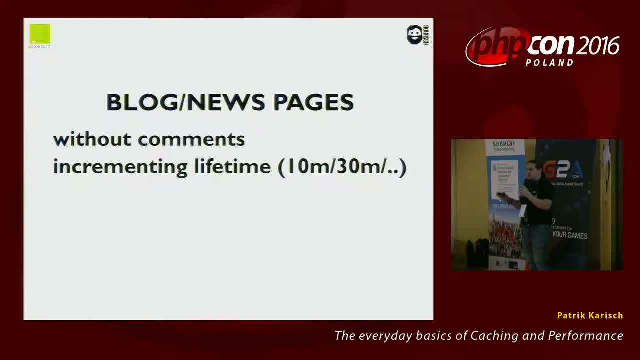 and the user can't see your fix because he has it cached in his browser cache. And I said: end it with a long lifetime. Maybe after a month you can set a lifetime of one or two days on the blog post And use validation. 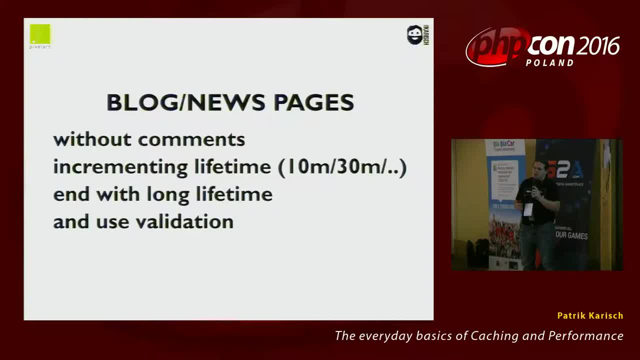 I said, if you have a lifetime of one minute at the beginning of the blog post, you don't want to have the traffic from the user again. you want to have only the if none match request from the user and return your 304 not modified. 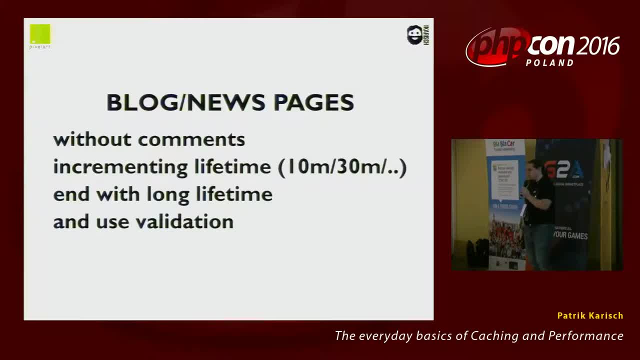 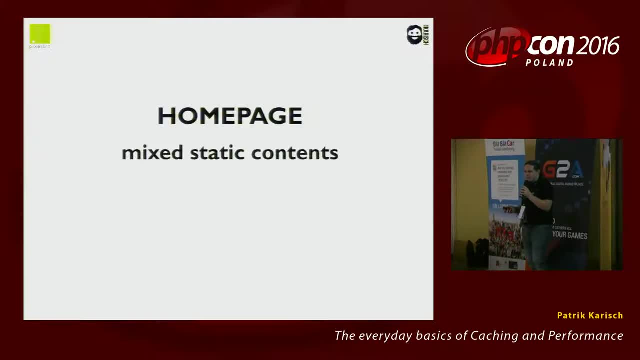 So you don't have traffic of the content. Another example would be home page, and the home page is really complicated to cache. It has mixed static contents and maybe you should only cache some lazy loading stuff for one or four hours or 10 minutes. 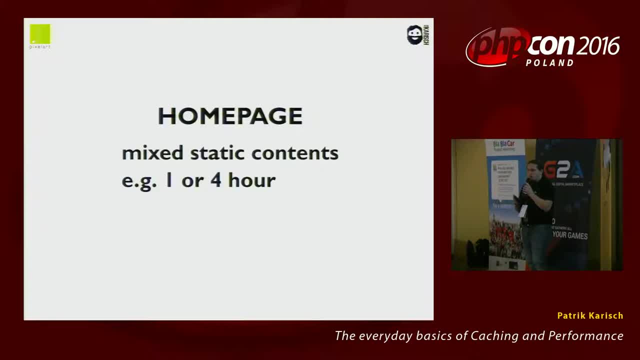 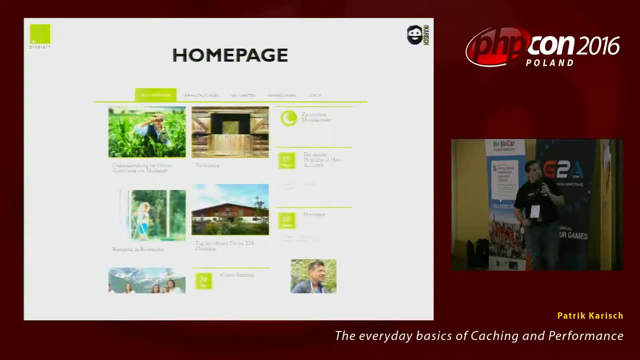 It depends really on the content which is on the home page And, if possible, use validation. This is a customer example. It's a dashboard composed of four different types of entities: Events, the main menu pages, blog posts. I even can't use ETEC calculation on this. 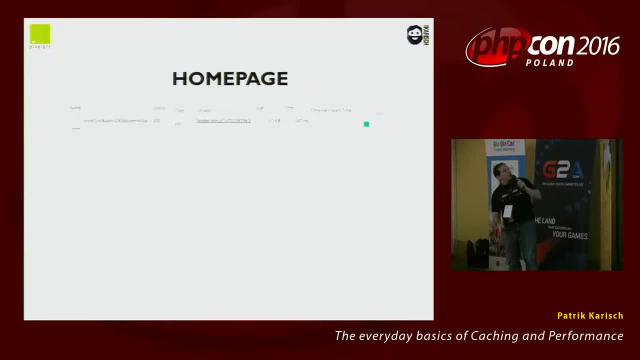 because it's so complicated. So let's look at the first row, If you can see it. we have a load time of 250 milliseconds. It's not slow, But it's too slow for a page where you still have 50 requests. 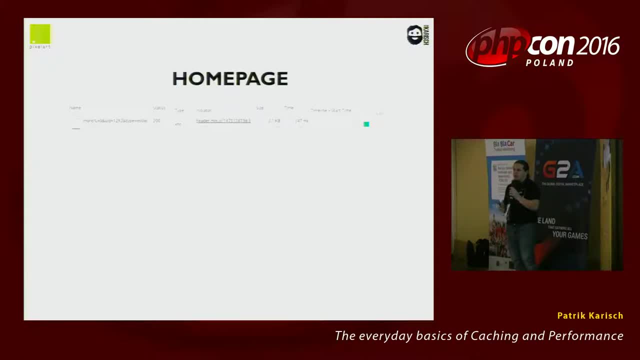 And 250 milliseconds is already improved because we have application cache which caches the whole output. So if it's not cached in the application side too, we have about two seconds. Okay, So if you send this cache control header with a max age of four hours, 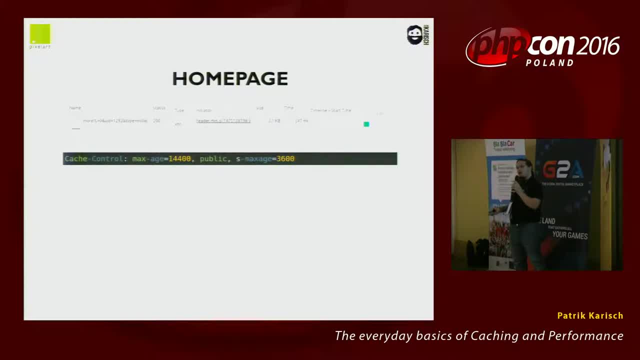 and we're doing a shared max age of one hour. with the proxy caches it's improved: only three milliseconds to load from the browser cache. And if you do this on a site where I have, for example, 20 HX requests, which are all contents- 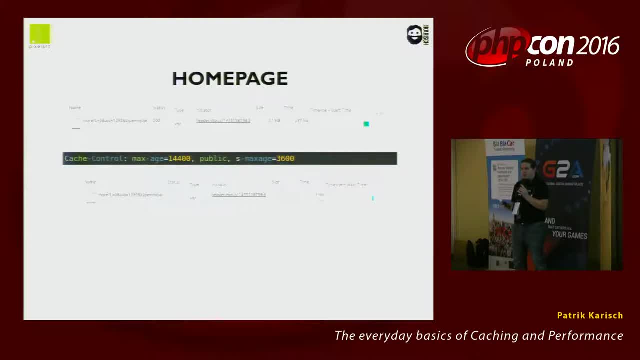 you can improve the subsequent loading times amazingly And your users love you again. And yeah, if the user presses F5, the browser sends a cache control max age with zero, which doesn't matter for your application, It's only an instruction for proxy and gateway caches. 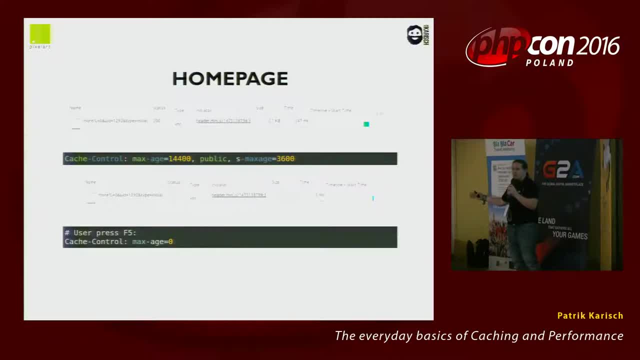 to refresh the content from the server side. So if I have a copyright proxy in between, F5 instructs your proxy cache to get the page from the server again. Okay, Maybe you have a map search on your pages: contact or retailer searches. 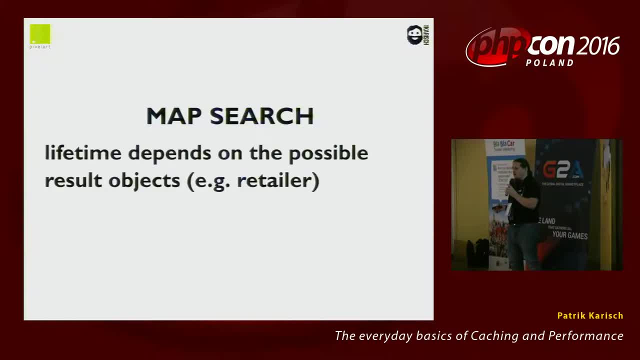 You maybe can cache these too. It depends on your object. If you have a retailer search to search for retailers, they will not change so often, so you could cache them And, of course, use validation. Always use validation, Article search or other filters like product searches. 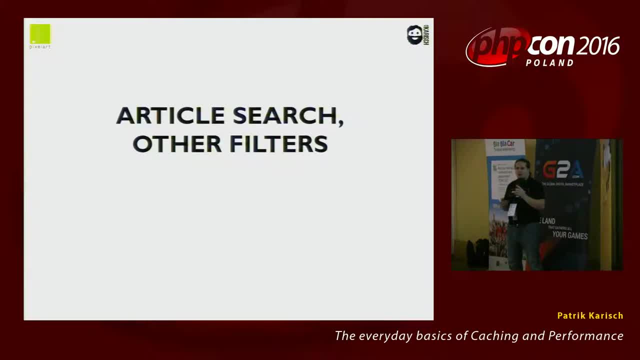 okay, products and articles are the same. whatever you can filter and search, please no caching. There are too much combination which would be cacheable and you don't have an improvement because the user changes filters and filters, so it doesn't matter. 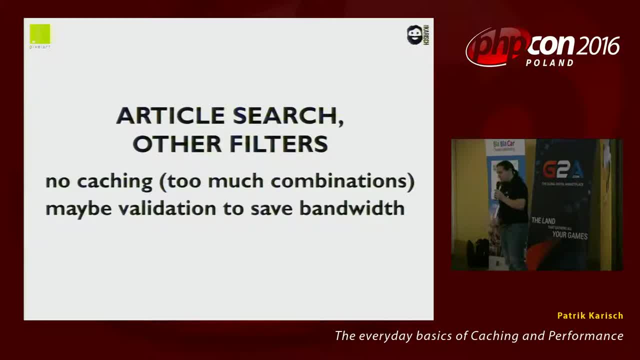 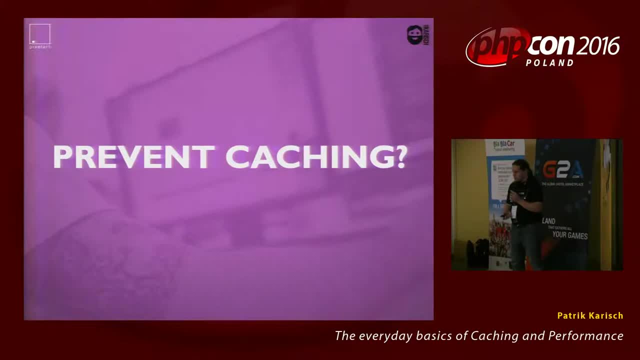 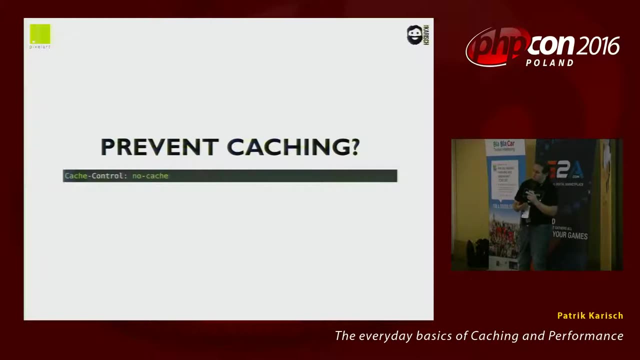 Maybe you can validation on the results And to prevent caching. sometimes you need to prevent caching, like in a checkout process. You could send no cache, but we have seen no cache already on eTech validation and last modified validation. If you don't send an eTech. 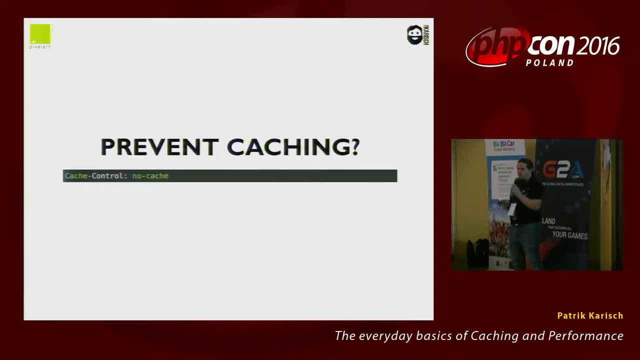 the browser should really not cache it, but not sure. If you have private data, maybe you add a no store attribute which should instruct the browser really to don't store this page. There's only one works If you're going through a checkout. 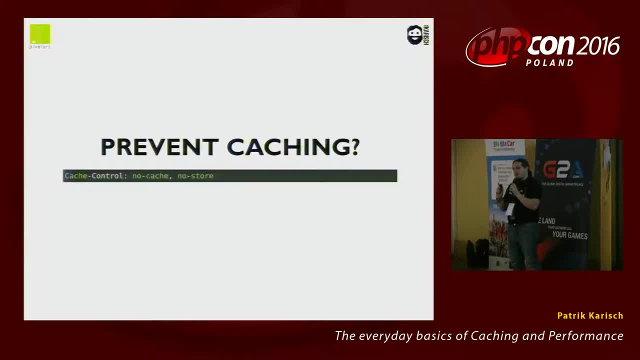 and the user presses back, the browser still gets the page from your cache, from the memory, when you press the back button. So please add mask revalidate, which really instructs the browser to get the page again from the server even when you press the back button. 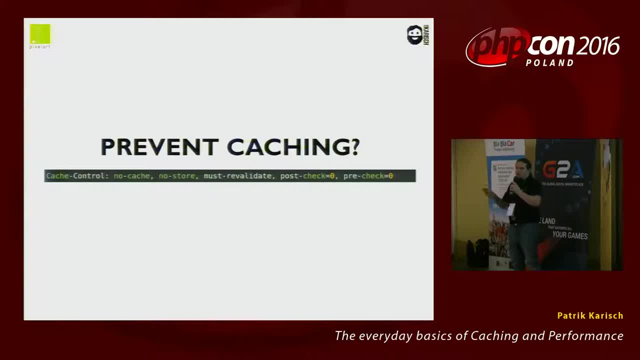 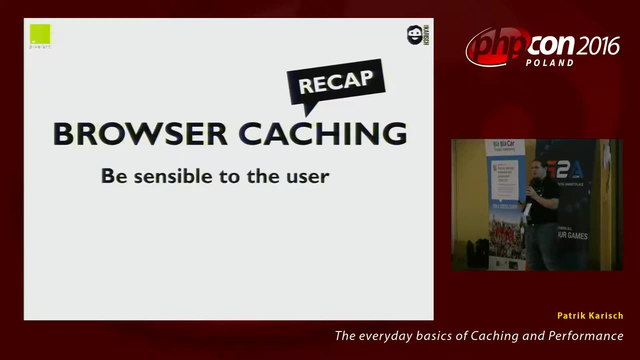 And at a post check and a pre-check too. I really don't know what they are doing, but I have seen them so often. if a site should not be cached, simply add them. Okay, let's recap this. You should be sensible to the user. 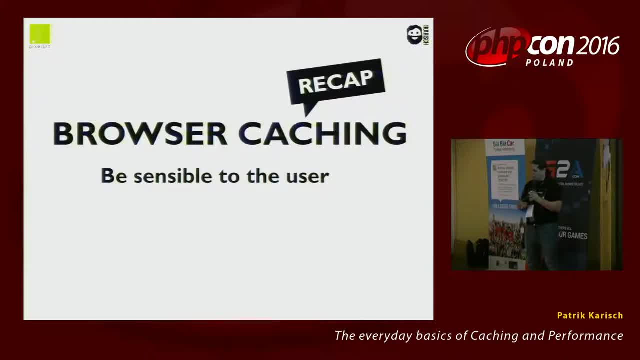 Get a good lifetime for depending on your objects, which means have a caching plan policy At the beginning of the project, work out a plan, a policy which objects could be cached with this lifetime and so on, And always have an e-tag on your responses. 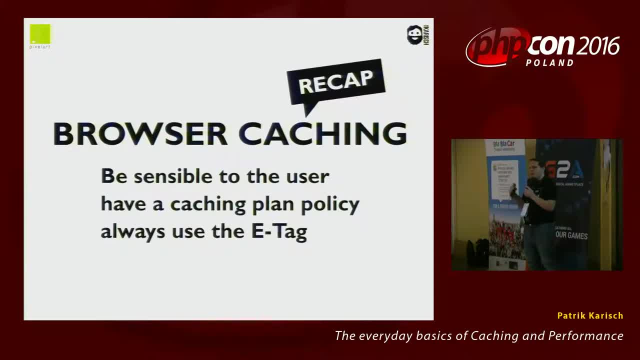 Even if you don't want to have the pages cached, have an e-tag because it can test on the server side if it's modified or not and can save the traffic of the response. And let's look at the cache plan policy. 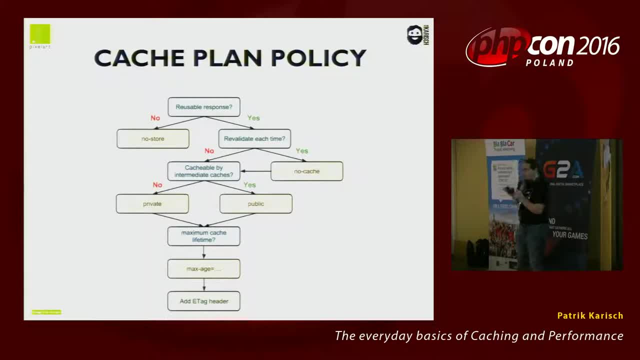 a cache decision structure. First you can decide: is the response reusable or not? If it's not, please do a no store like checkout process, my order's history and so on. If it's reusable, you have to decide: should the browser revalidate it each time or not. 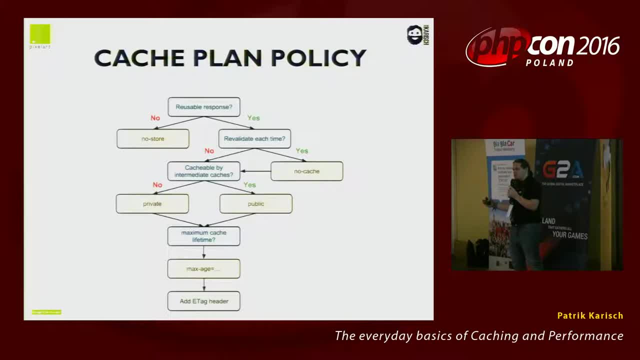 If it should be revalidated, set a no cache together with e-tag or last modified. If the browser should not revalidate it each time, simply add a max age. and first you have to decide it should be public or not. And, as I said, 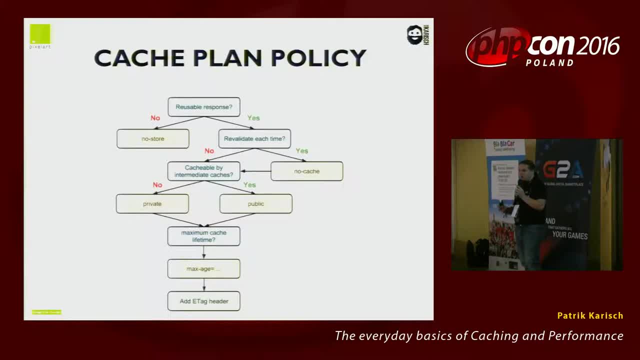 please care about your user privacy and user data, which should be cached, should always be private. And then you set the max age and even if you have a max age still set the e-tag header to have validations after the max age is over. 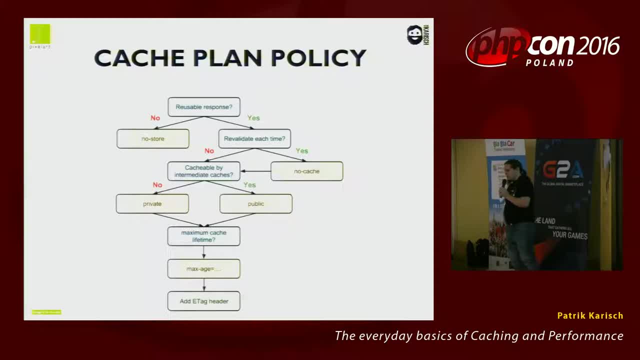 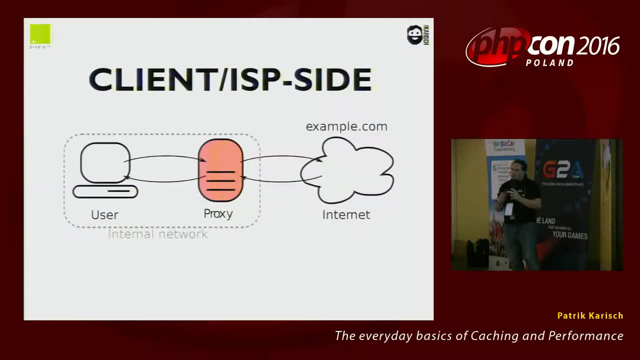 and the entry is stale in your browser. Then a sneak peek to proxy caches. The proxy caches are on the internal network or more on the client side. It depends if it's a corporate proxy in a company or it's at the ISP at your internet provider. 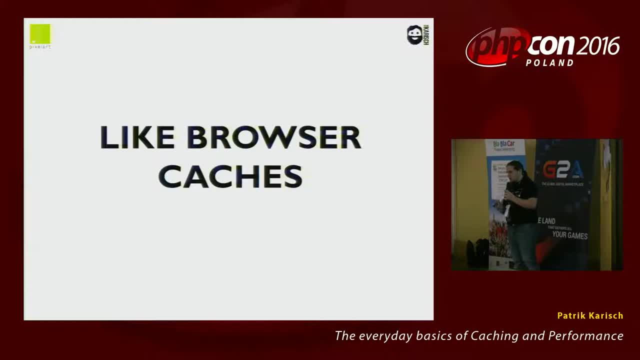 They behave like browser caches, but they are shared Like in a corporate, in a company, they are shared between all employees At the internet provider. the cache is shared between all customers of the internet provider. They are still URL-based, but they are really annoying. 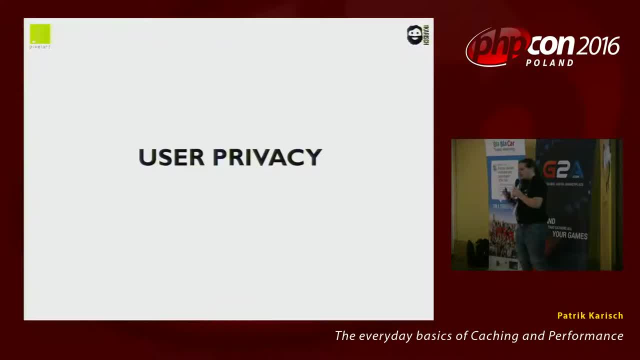 because there are some cave-ins. As I said before, the user privacy Care about if your response should be public or private. I cannot say it often enough, And proxy caches don't behave often like the standard says. Maybe there's a company proxy. 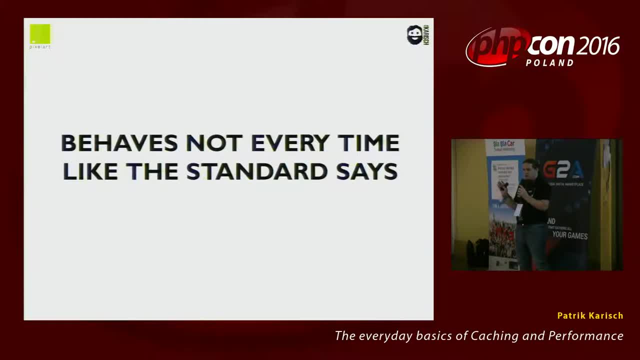 which wants to cache everything, even if it should not. Shit happens. but then the customer says you have fucked up, but not the admins. And maybe there are mangled headers from proxy caches and even antivirus software installed on the user's computer. 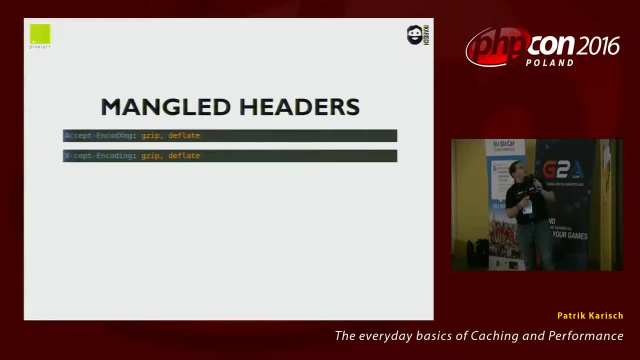 like accept encode, xing or accept encoding or all x or all minus or all tiled. This can encounter on like 5% to 1% down of all your users. It's not nice So you can't compress your response and your traffic increases again. 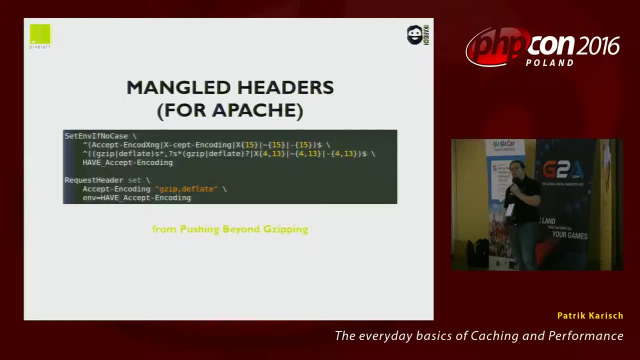 To tackle this, simply copy the snippet in your Apache config and this regex matches all these mangled headers and if it finds one, it sets a regressed header. to have a clean accept encoding, Simply copy it. It doesn't matter if you have a user base. 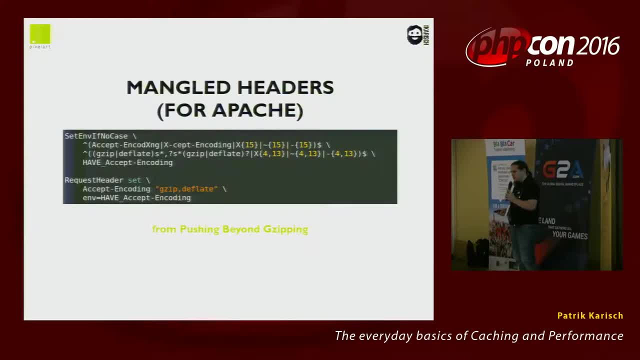 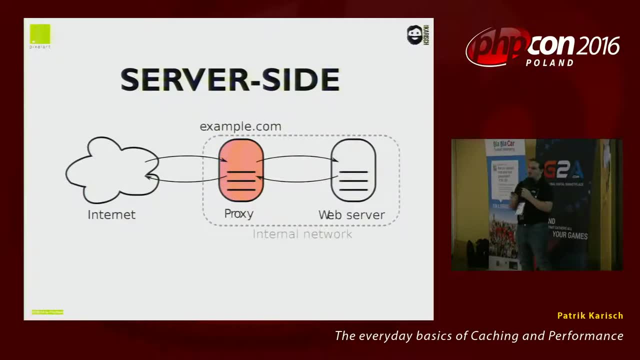 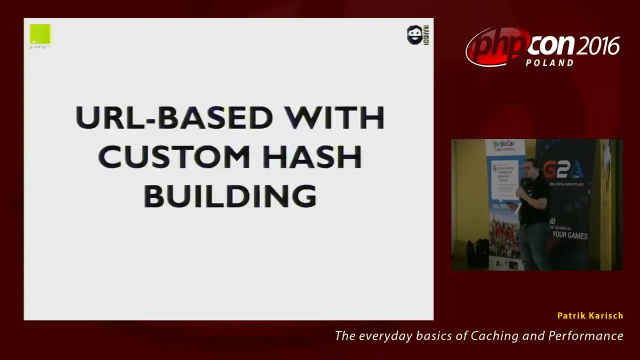 which has these problems with mangled headers or not, And then the gateway caches, or better known as reverse proxy. This is again on your side. It's not directly in your application, but you have still full control over it. You can do a URL-based caching strategy. 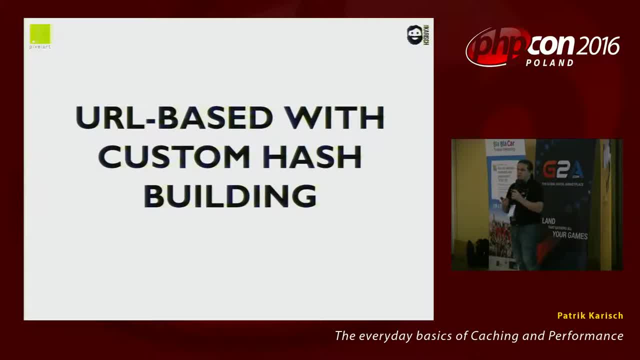 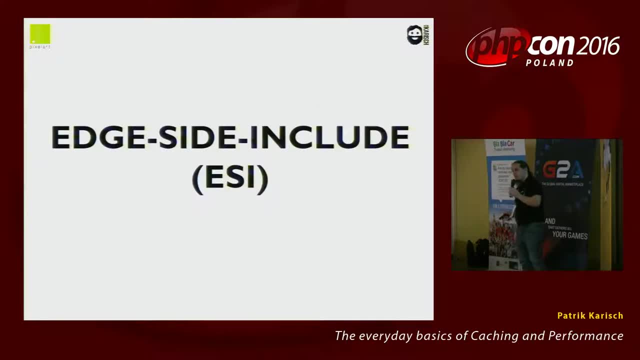 together with a custom hash calculation. This custom hash can depend on any regressed or response header, or even on cookies, which should be filtered. And the pro of a reverse proxy on your side is you can do. edge site includes, which means, for example, 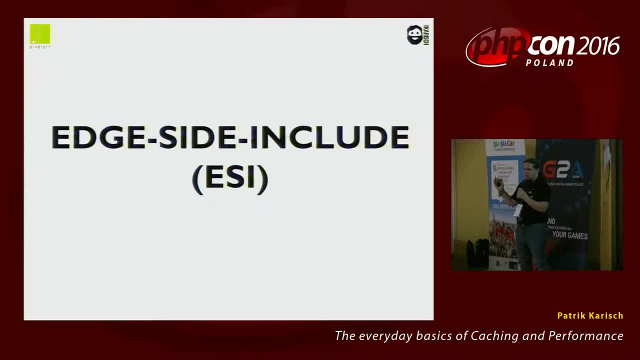 if you have product detail page. the product detail page should be cached for one day or a whole week, but not the price on it. So simply set a tag where the price is ESI include to a backend route for article price. 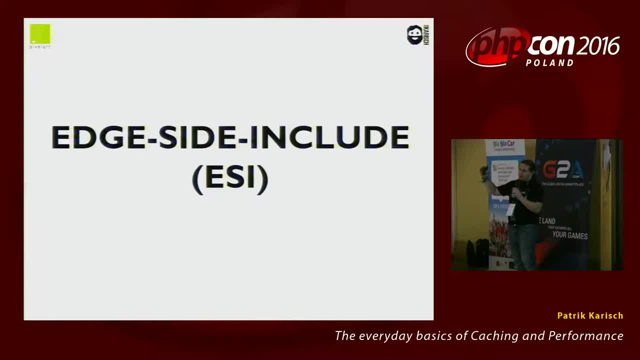 and then if the user hits this product detail page, the reverse proxy cache can- Sorry- get lost again. This reverse proxy can get the page from the cache and then it sees the ESI include and fetches the price live from the backend. 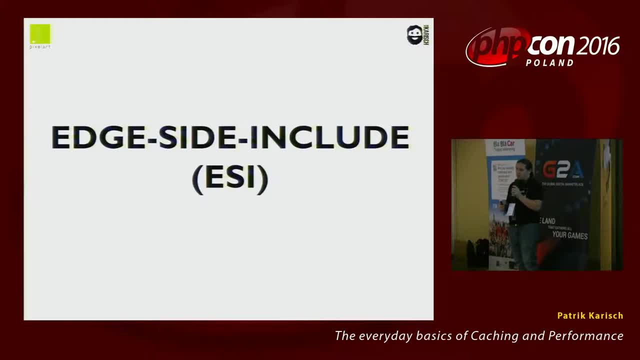 And now the user always gets the actual price and not a cached one, Because don't have a cached price at the user. He wants to buy it, puts it in the basket and then have a different price. He's angry, he's annoyed. 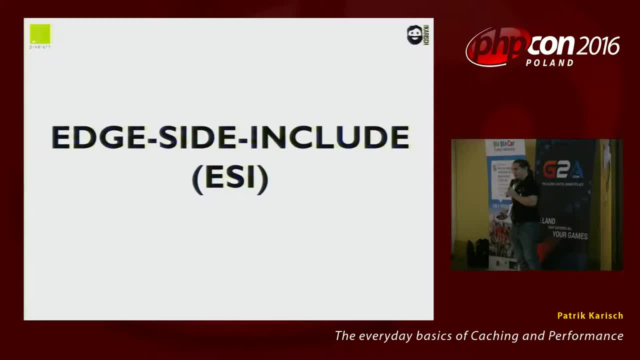 and it could be a legal problem too. Then the bad part about using reverse proxy is you have a complex invalidation. You need to use ban requests, flush requests, and there are only two hard things in computer science: Cache invalidation and, of course, 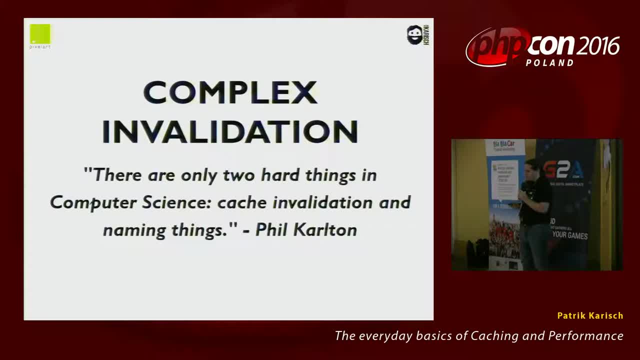 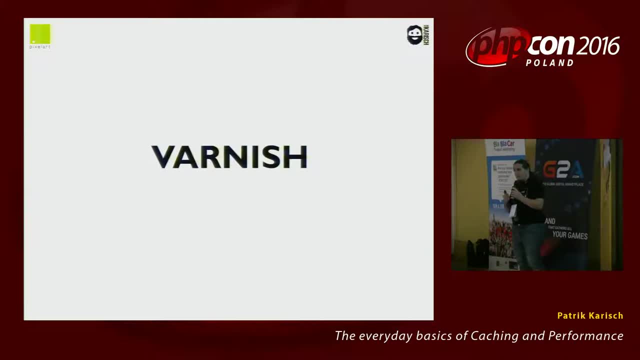 you have to do the same things. It's a nice citation by Phil Carlton. If you want to use a reverse proxy cache, either use varnish, which is the most advanced one. A bit complicated configure. For simple sites you could use engine X. 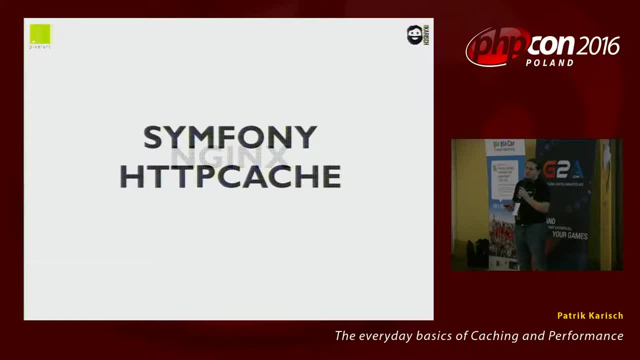 if you're not using a patcher, Or at least you should use the symphony http cache component, which behaves like varnish but uses a file-based caching. Don't go on production without a symphony http cache If you have a symphony application. 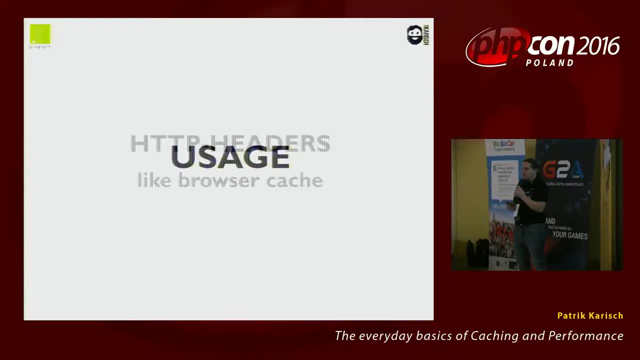 The usage for this reverse proxy cache is the same like a browser cache with http headers but, as I said, you have extra requests for banning and flushing cache entries. You can't simply do this cache remove. You have to do a request to the reverse proxy server. 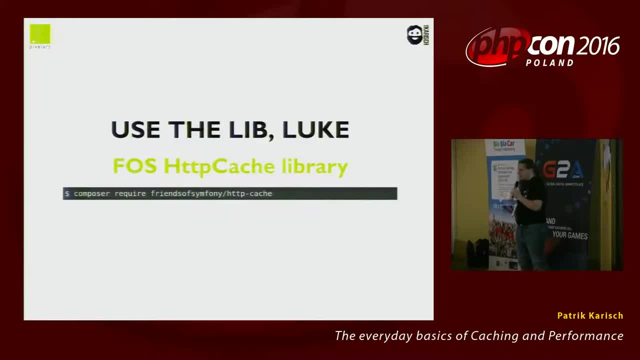 And, for the sake of it, use the lib again. Use the false http cache. Also, if the vendor name says friends of symphony, it's a standalone library and it has an actual symphony bundle. So if you ever are in need of a reverse proxy, use a lib, Don't do the curl request or guzzle request on your own. And there are also common mistakes. while using a reverse proxy, You didn't clean up cookies, For example varnish, in the default config if the browser sends a cookie. 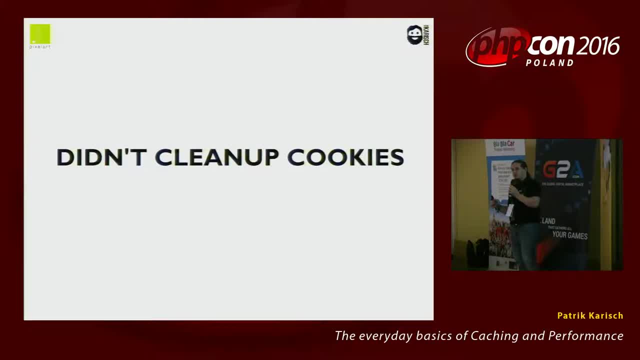 it wouldn't be cached. So you have to clean up cookies and maybe have one or two cookies which are used in the hash calculation and forwarded to the backend and then decide it's cached again. And please don't cache user-specific content. Don't cache the credit card data. 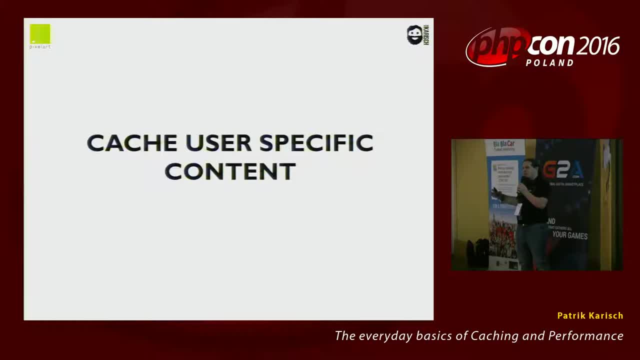 of a user in your reverse proxy. Otherwise every user will see this credit card data And wrong cache headers. It's the same as before. If you send public to a private request, it's the wrong cache header And unsafe requests. 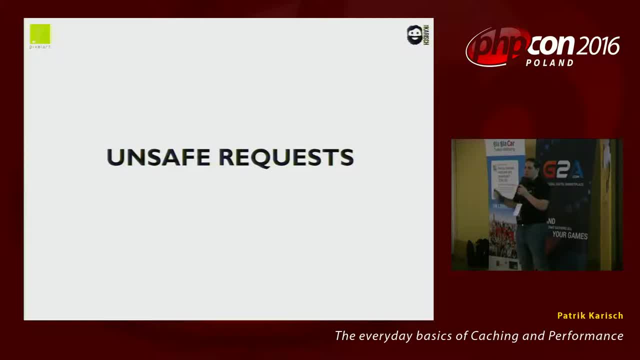 And unsafe requests is all those requests which are modifying data, Post put etc. For example, varnish. again In the default config it won't cache any post requests. If you have an error in your config you may cache post requests. 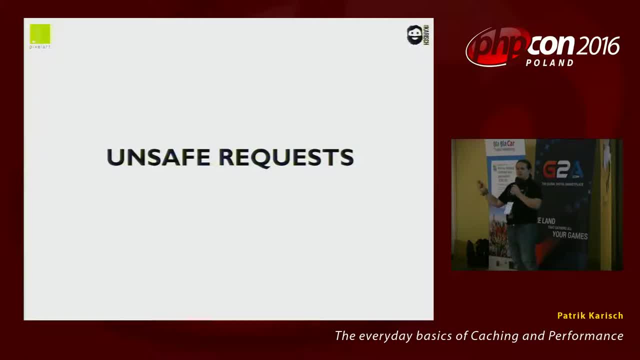 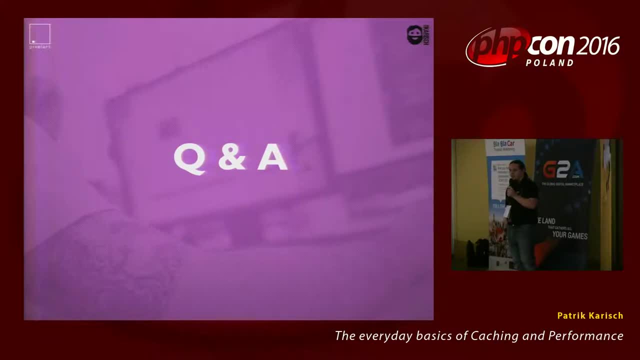 And that's bad. So to be friendly to our camera guys. that's the end And the time for your questions. No questions, Hi, thank you for your presentation. I have a question about setting the cache for Symfony response. You show us some methods like set max lifetime, etc. 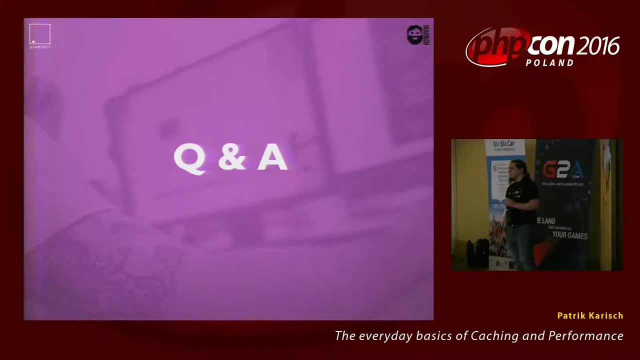 So I have a question: How do you handle when you want to turn off the cache in the Symfony application for developers? So the cache is cool for production, but how do you turn it off for developers? If I understand you correctly, you mean the Symfony HTTP cache component. 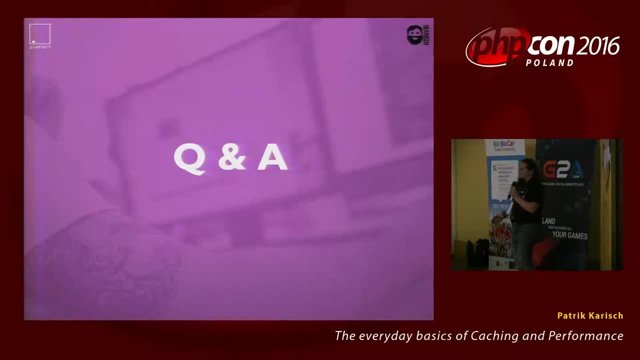 Yeah, yeah, HTTP foundation response: No, the HTTP foundation is different from the HTTP cache component. The HTTP foundation, the response object, is by default not cached, So you always have to do set max age or anything else to have the response cache.